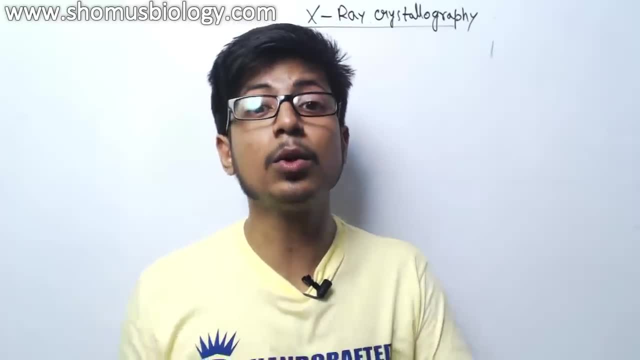 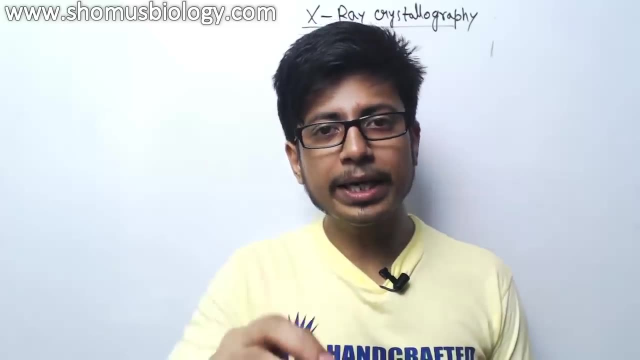 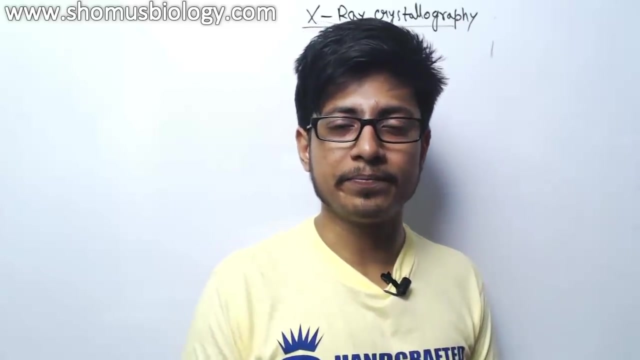 molecule. It could be a chemical compound, any organic chemical compound, including the macromolecules of our life, for example proteins, nucleic acid and stuff. So we can identify the structure of those unknown proteins or nucleic acids, For example, say, the DNA, the deoxynucleotide. 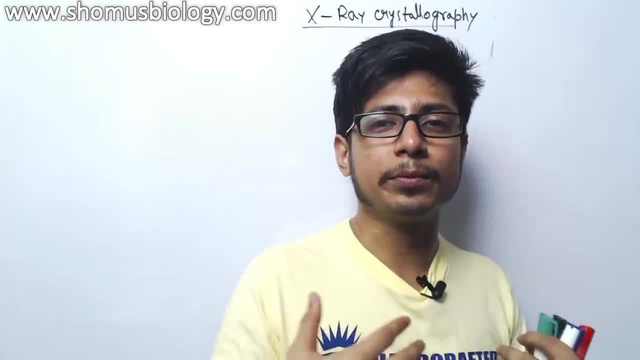 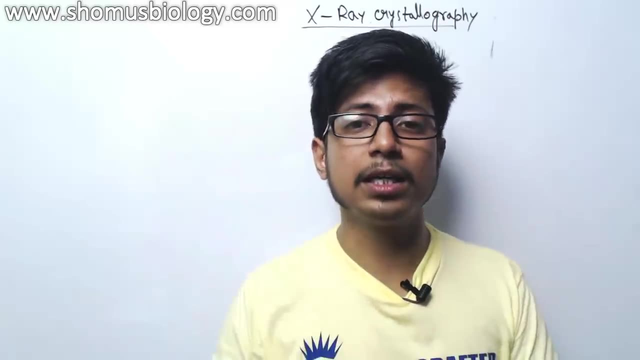 the DNA. the DNA structure is determined using extra crystallography at the very early point. That is going to give us an idea about how exactly- whether the DNA is spherical or or like spiral. that's going to inspire us to find out the structure of the DNA. So let's look at here. 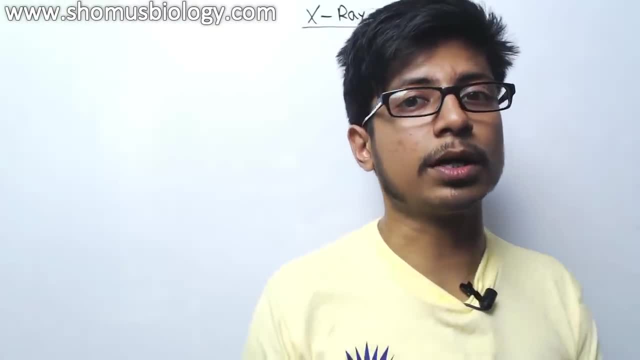 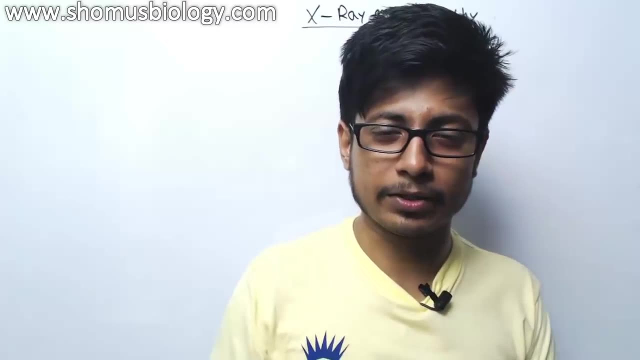 the overall process of extra crystallography. That's what we're going to talk about today Because, you know, I find many videos and many people understand all those critical formula and stuff about extra crystallography, but they lack in the idea of what, the concept of what is. 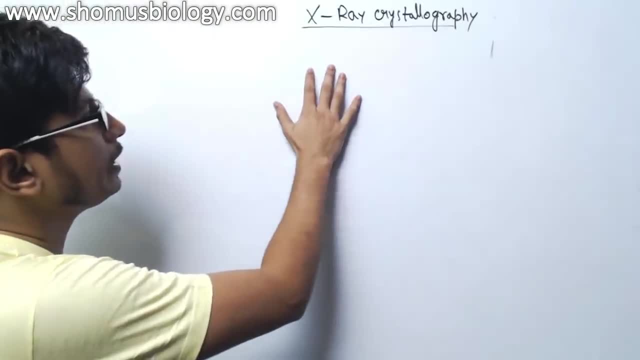 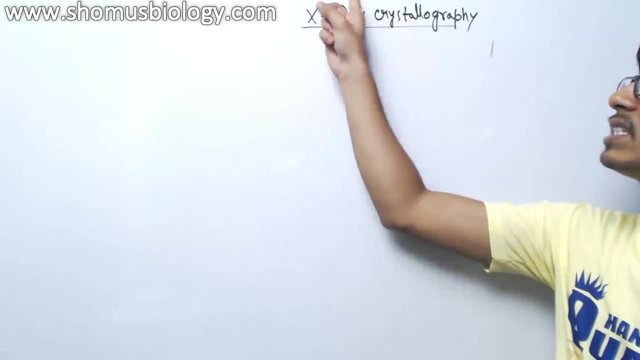 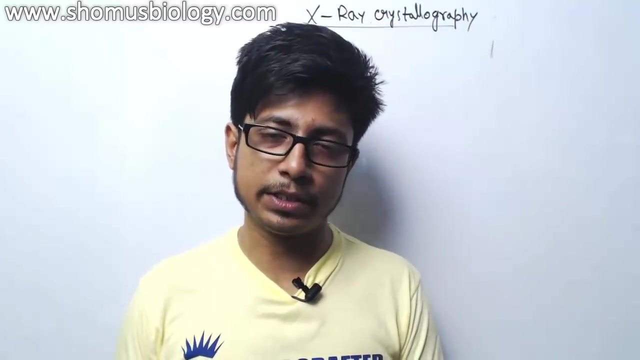 crystallography in overall sense. Now, extra crystallography is performed only to crystals. Why so? And in this case we use only x ray instead of any other light, because we can. we cannot use normal radio wavelength light, the visible light that we see. we need to use x ray because we're dealing with here the molecular. 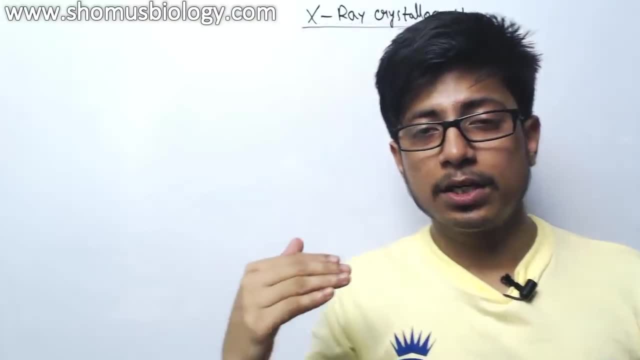 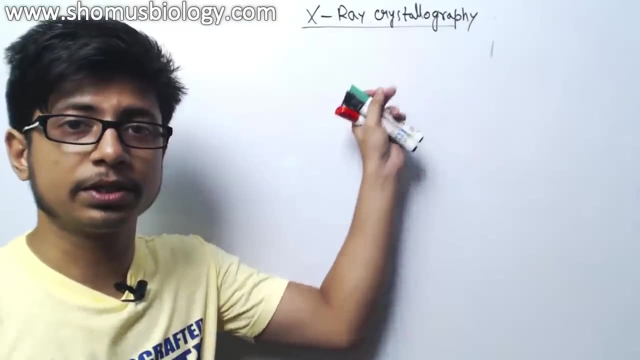 structures, the structures in the very atomic level. that is not determined, that can't be determined with the visible light. that's why we need to use x ray And why we use crystal for the crystallographic process Now, in any molecule. if you want to see, you need to put it in the crystal format: crystal format. 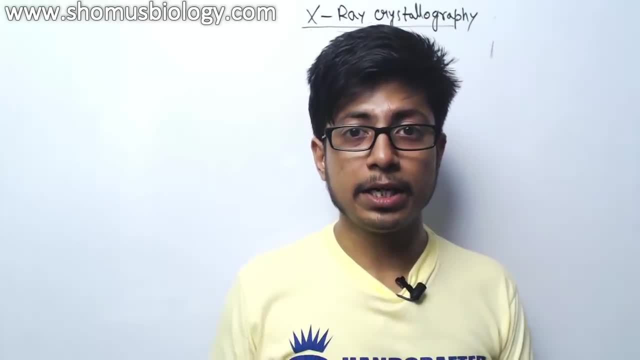 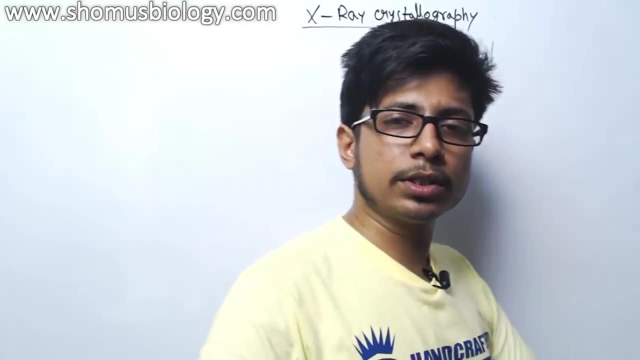 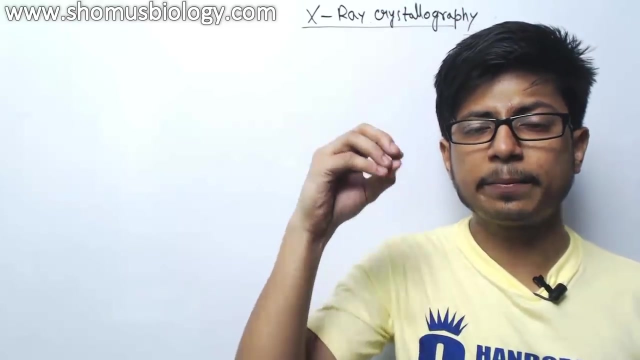 by cooling and condensing that compound that we are trying to find the structure of. Now, why we look at the crystal? because, remember, normally all those molecules, these organic compounds, or the all those macromolecules, whatever we are talking about, those molecules are not stagnant, they are present. 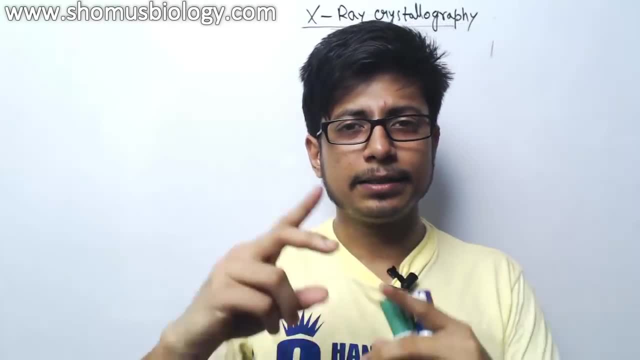 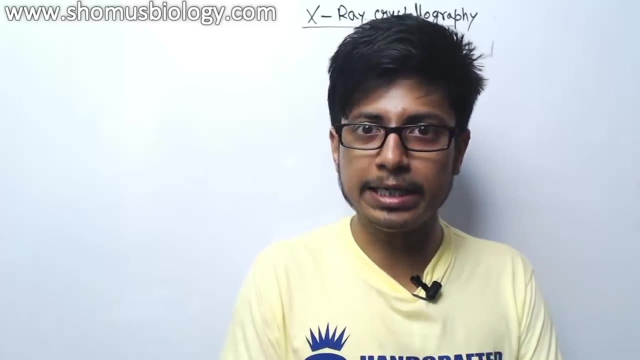 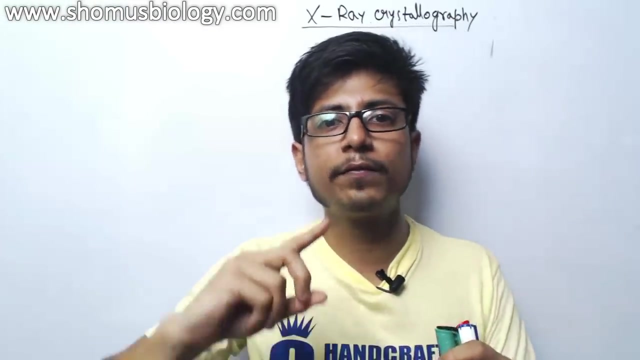 in different orientation. I mean they're moving, the bonds are changing with the time, it's rotating and all those things are modified from time to time because that's for the living organism. That's true, they're changing over the time, But it's very difficult for us to identify a molecule structure if all. 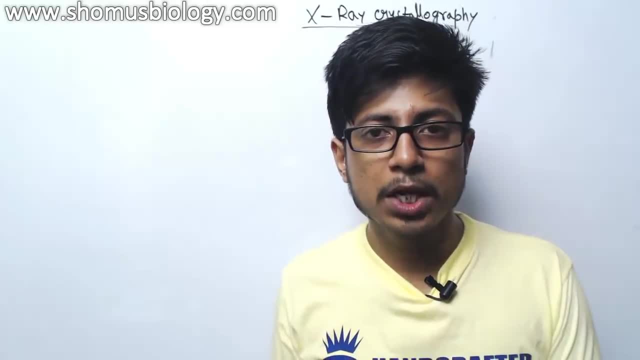 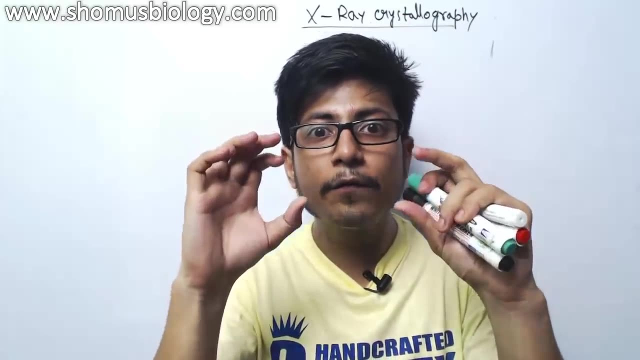 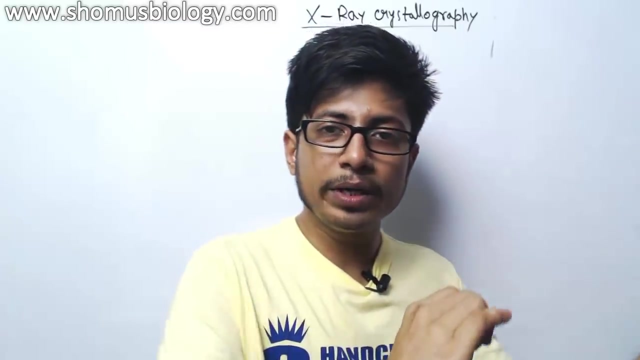 those bonds are changing, rotating and modifying. So the only way and the easy way to get the structure is to make that whole molecule freeze and fixed in a point that we can achieve with forming a crystal of that molecule. Once we make the crystal we can be sure that that molecule that we made the crystal of, 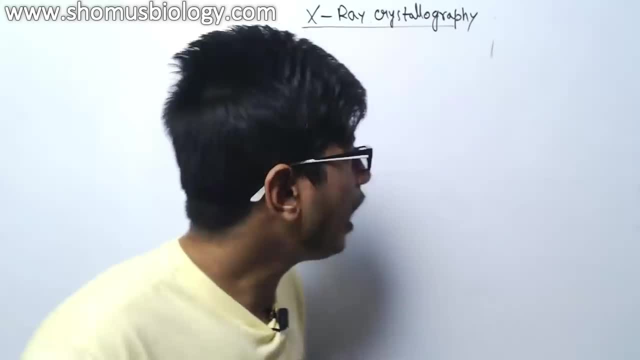 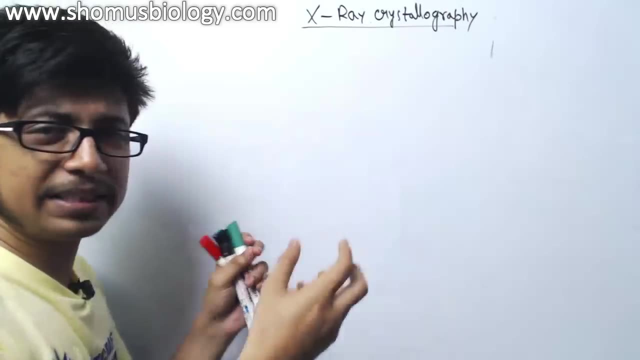 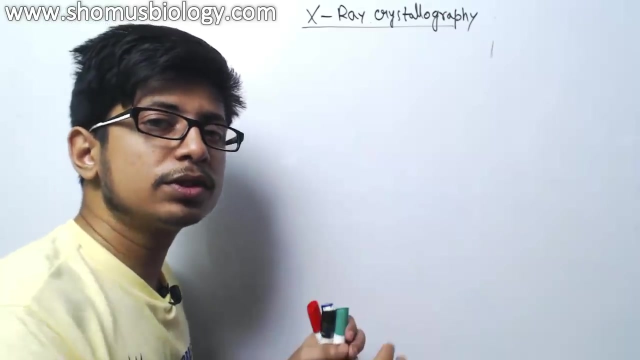 that is fixed, that is permanent, that is stagnant. So now, once that molecule is stagnant, they have a different type of atoms, different type of atoms linked with that in different regions, and that will be fixed throughout the experiment And from the beginning to the end of the experiment we use the same region of that. the same same atoms are present in the same region of that crystal. 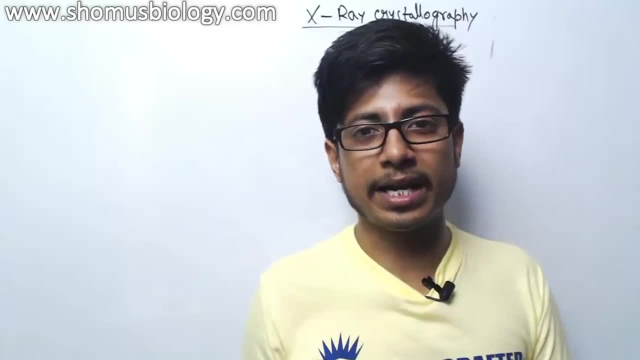 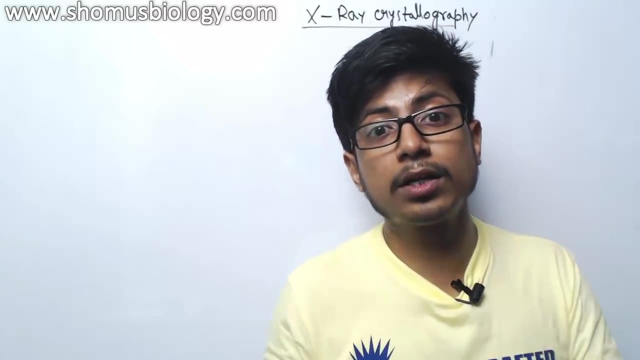 So it's very important for us. it's very easy to identify that the target molecule structure. That's the thing Now for those type of molecules which we cannot convert them into crystal, we cannot use them for extra crystallography. 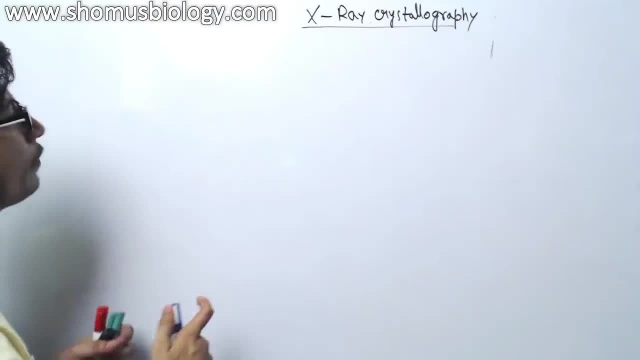 Okay. so let's look at it As I told you that we can form a crystal with it, And for the crystal means we are talking about 3d structure here. So if I draw a 3d square like this, let's say this is a 3d square, the structure 3d. 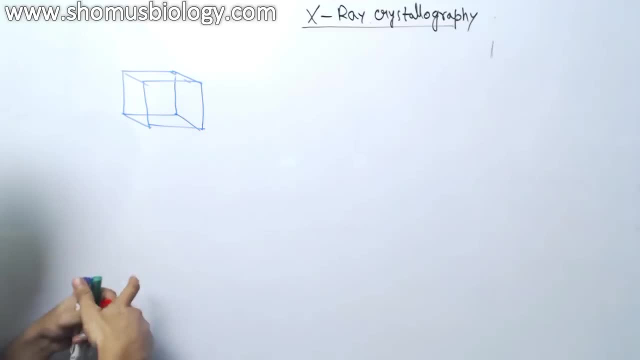 This is a crystal, for example, and there is a molecule. there's a protein molecule that we are going to look for In 3D dude. it says a 3d dimensional space. there is a protein structure over there, For example. 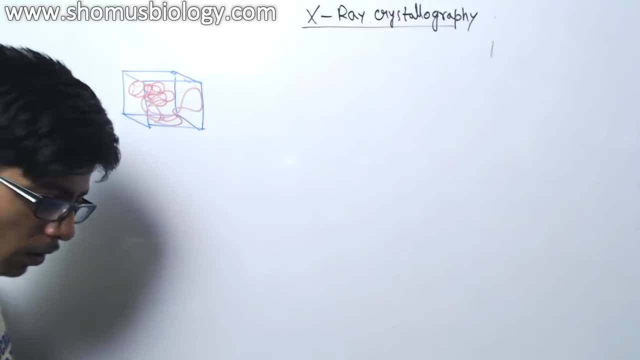 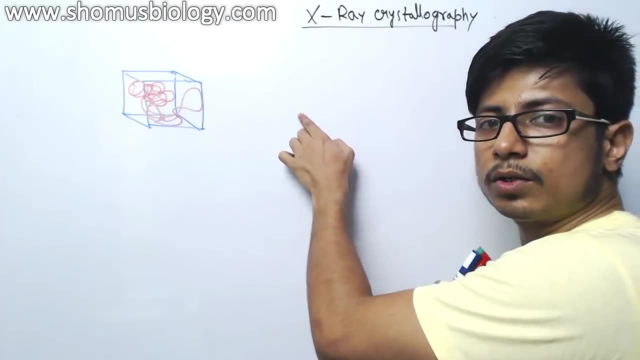 As you see, the protein structures a different way. it's not touching the overall crystal, but this is how the crystal looks like. Now the idea of extra crystallography, the very basic idea, is we we put X ray to interact with this crystal. whenever we hit X ray to the crystal, 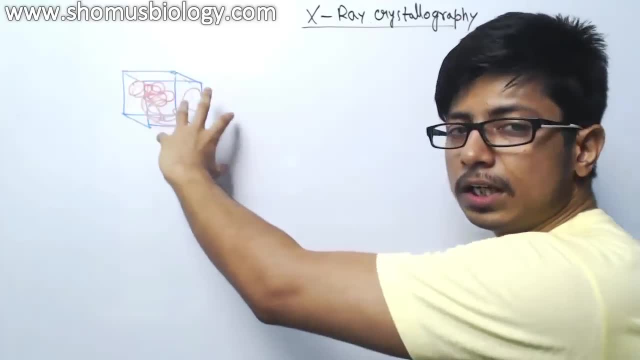 This crystal will diffract. The part of this x ray diffraction means it's very similar with the reflection. So this is the chest of gyros crystals, cartyond audible. This is pussy. A glass p segregation ad the 휴�duke window, and so on. 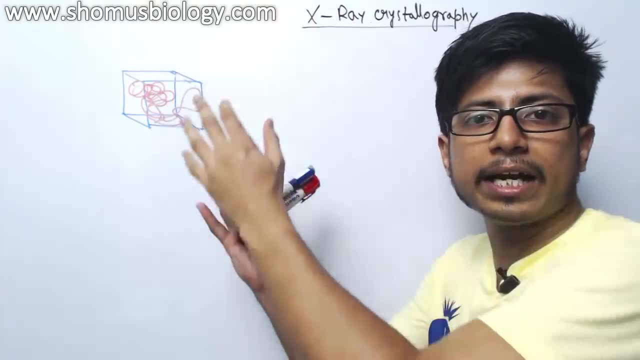 No quarter per beatisc, twenty four percentee. you can see left parts, one terminal, left and right, half per stack and two zadifiers He's find right behind the letters 297.. that we simply change, and change the direction of the angle that the X-ray hit this crystal. 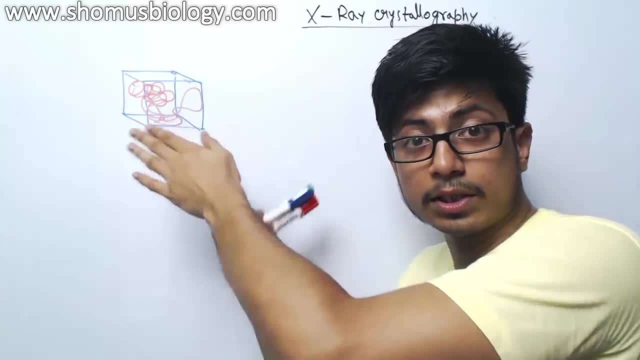 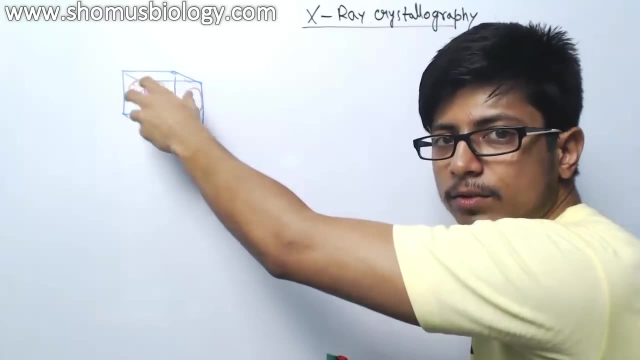 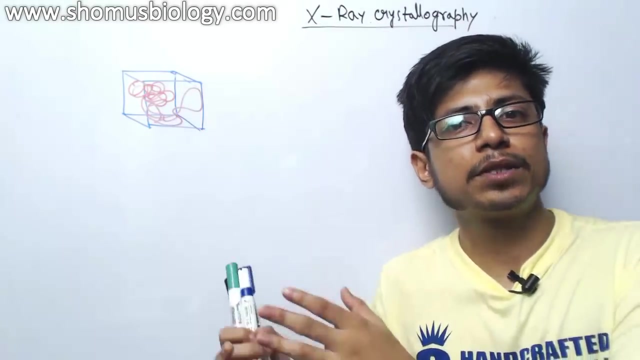 So X-rays going towards the crystal. it's interacting with the crystal and it is diffracted in a specific angle. right now depends on the type of molecule that we're looking for. the diffraction pattern varies and this diffraction pattern is unique for different types of molecules. 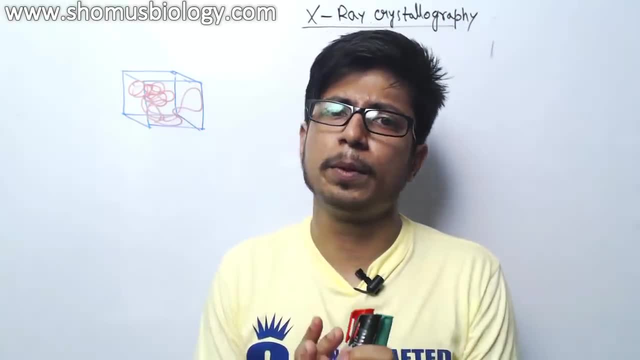 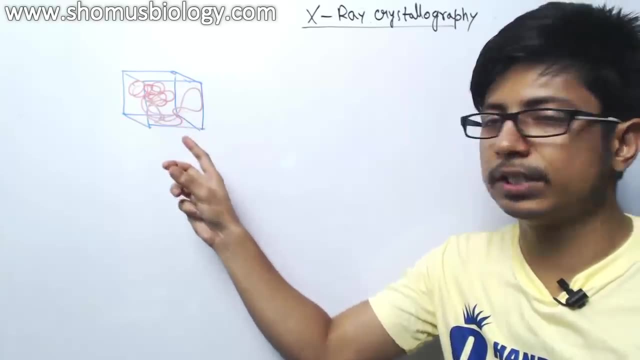 that. so we understand if the molecule is more complex will be more different varieties of diffraction. that we will see simpler molecule with very less region, which are most most region of the crystal. if it's blank, that it will give us less diffraction. that is the 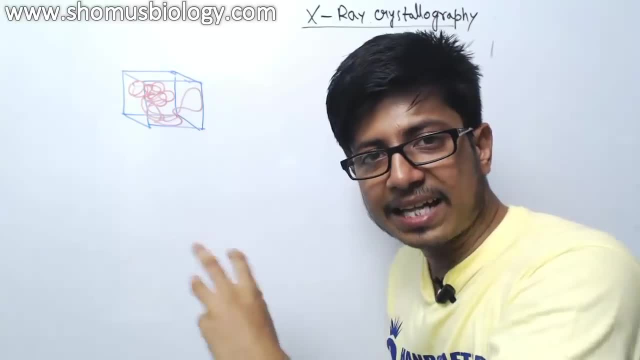 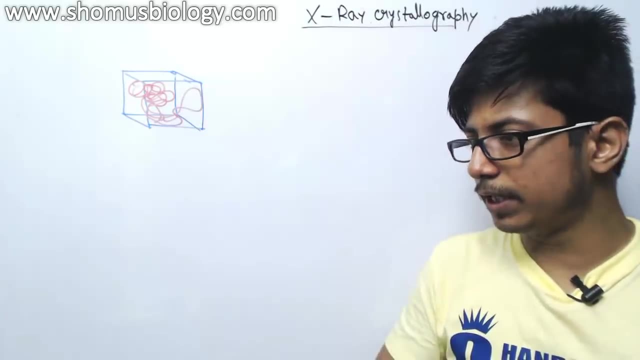 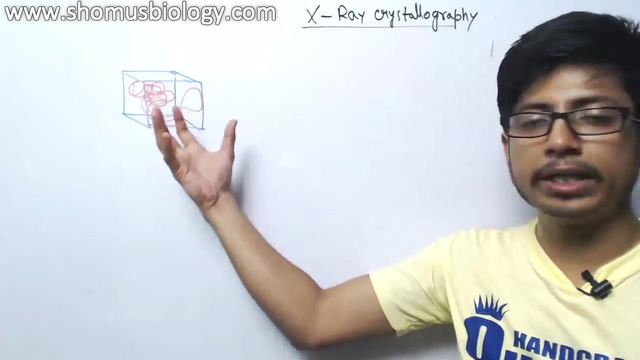 whole idea. we will get the data from the diffraction and that data is going to help us to find out about the structure of that molecule. now let's say here, as we are from the biology background We want to talk about, Are guessing and identifying a structure of a protein. so let's say, the protein we make. 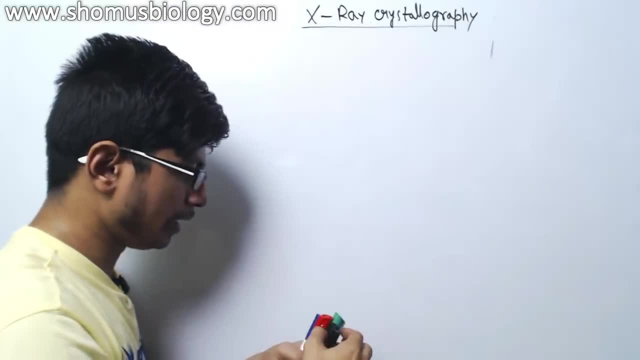 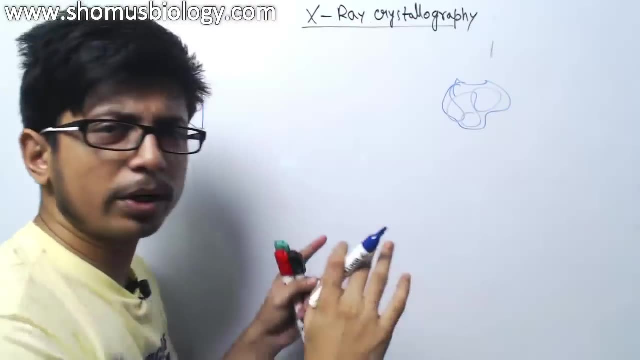 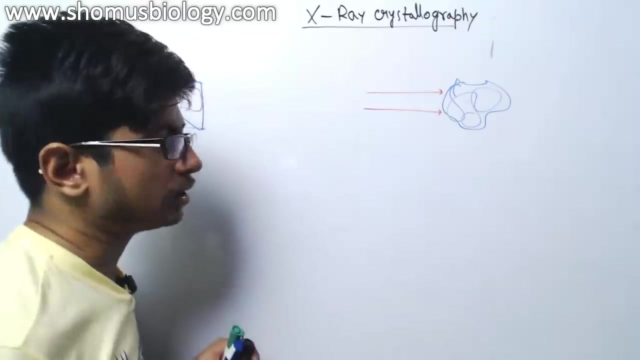 a crystal of that protein. so we have the protein crystal in our hand. So let's say here, this is a, this is a protein crystal. I'm not drawing the geometrical shape here, but the very simple idea is we are applying the X-ray crystal is getting different and 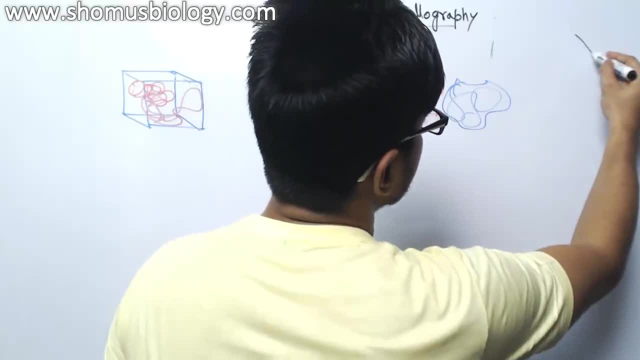 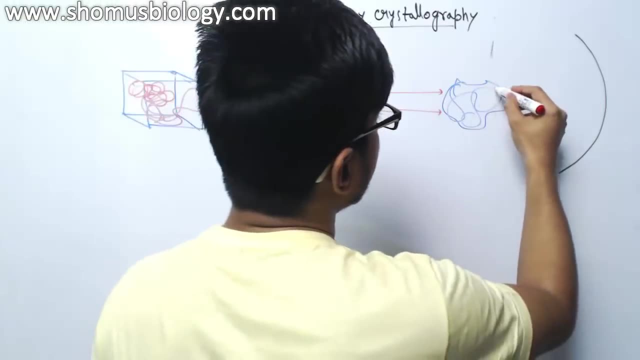 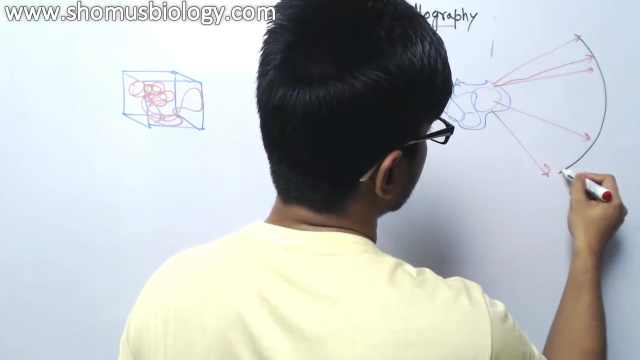 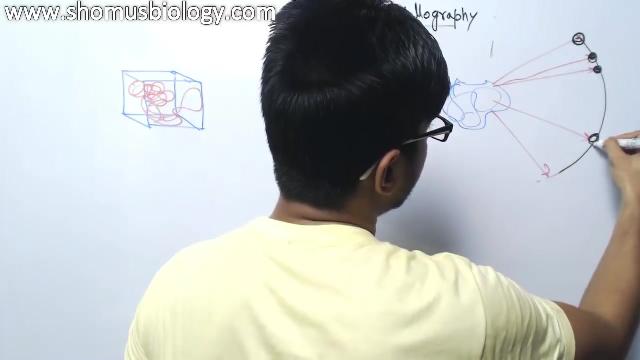 we also have a detector here at the end, The X-ray film, where we can see the spot after the diffracted rate. so say the diffraction, one diffraction, go there, another one goes there, goes there, there, there. so there are different diffraction. so if you see this X-ray film will see a diffraction pattern wherever. 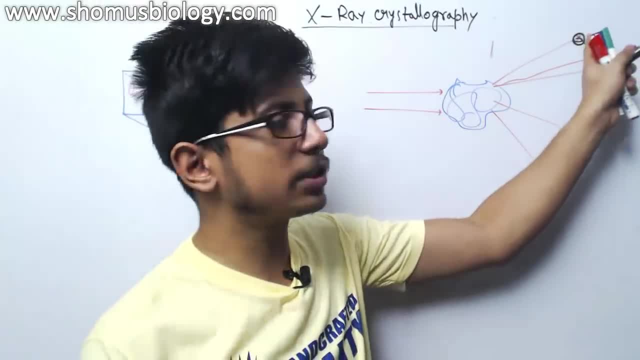 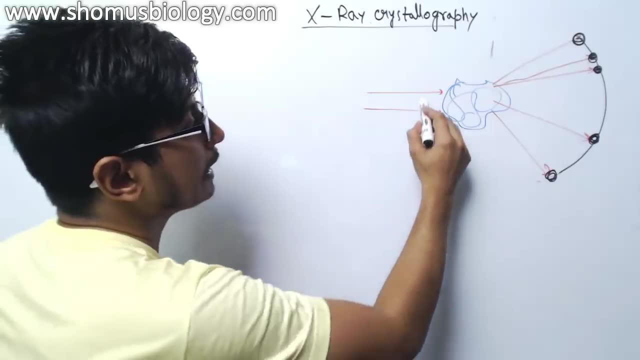 there is a X-ray heating, that film will have a different spot that is generated in that thing or plate. that plate is very important to find out, Find out, Find about exactly what kind of protein structure that we're looking for now, if I say this is. 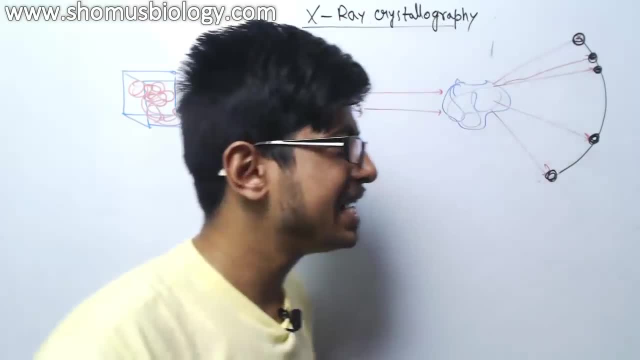 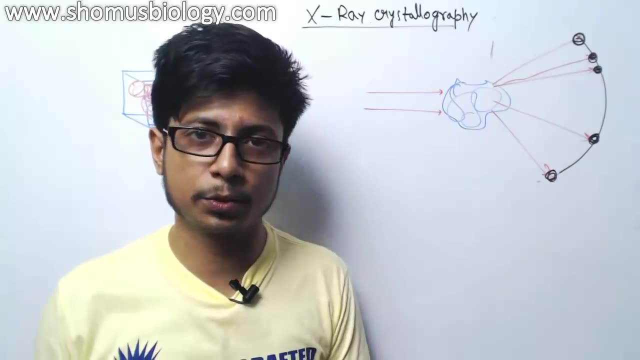 not that simple in that idea, because a protein is very complex macromolecule. it is filled with so many groups, so many subunits and many things are attached with each other. and once you're looking at a crystal, as it, as I told you here, just look at here, it's a geometrical 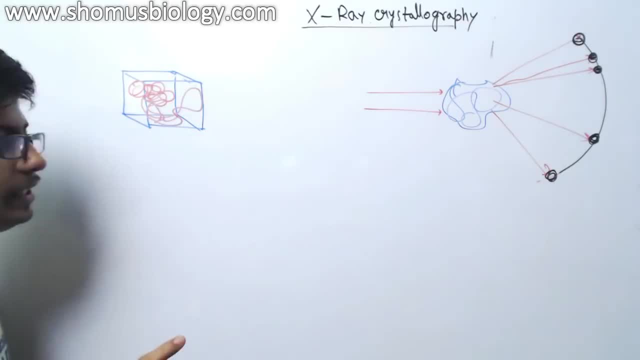 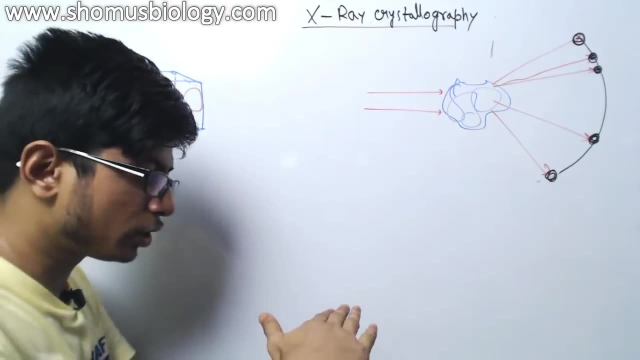 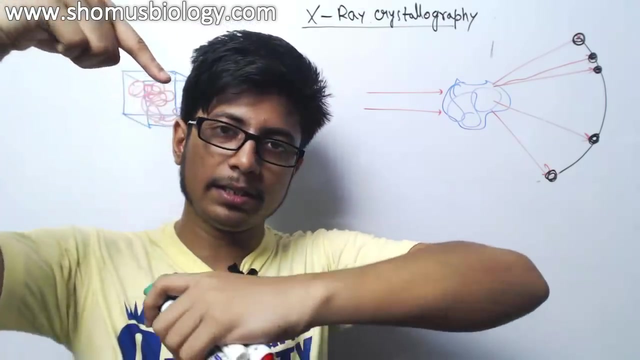 shape. this is a three-dimensional shape and the idea is X-ray will come And X-ray will be diffracted. that means there should be a plane for the diffraction. if you think about diffraction in overall process, it means it's very similar with the reflection. 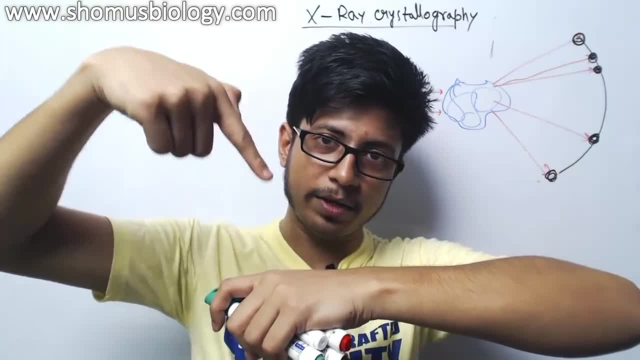 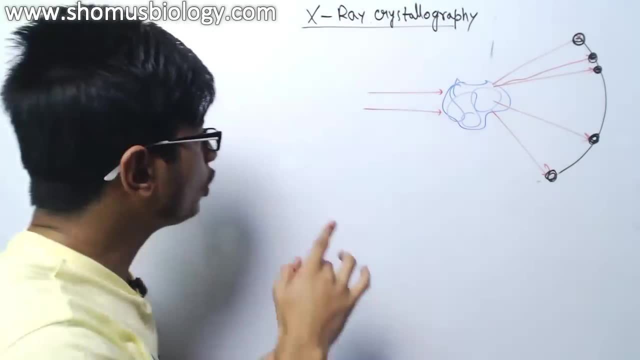 so there is a light comes in, or or a ray comes in, a wavelength comes in, it hits a specific plane and reflected away. that's the idea. so the diffraction that we want to see here is due to different planes In that crystal, In that crystal. 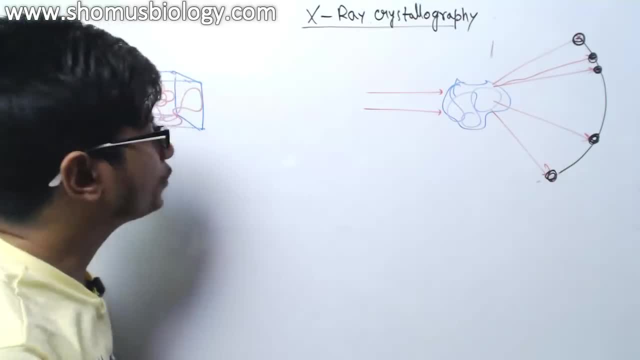 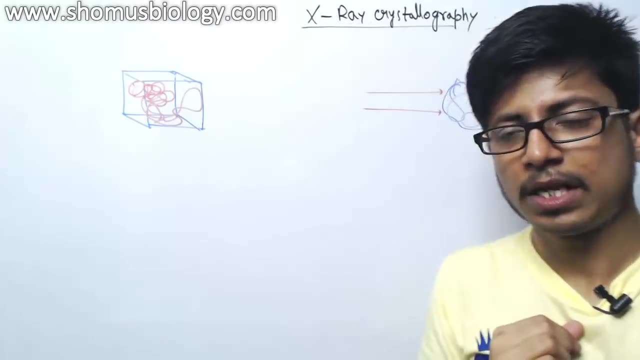 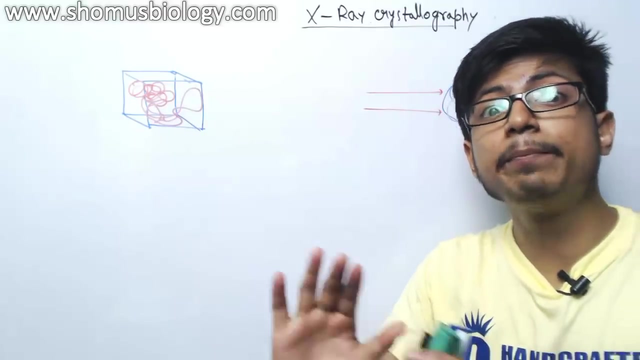 So what we do is we take the big crystal and we break it down in smaller unit fragments. so let's say we take this crystal for this whole protein. we break them down in smaller fragments- which are imaginary fragments, by the way. we we are not actually breaking the. 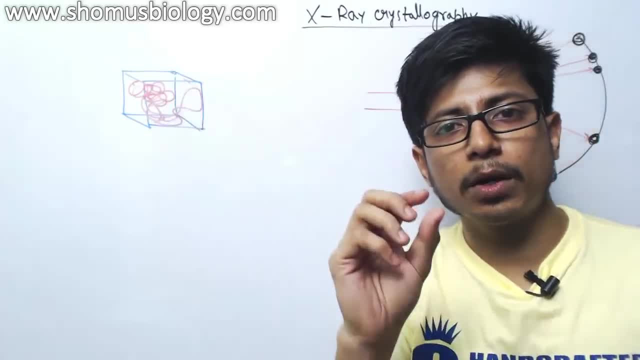 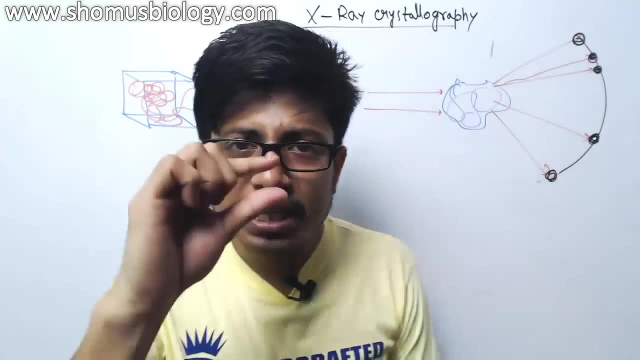 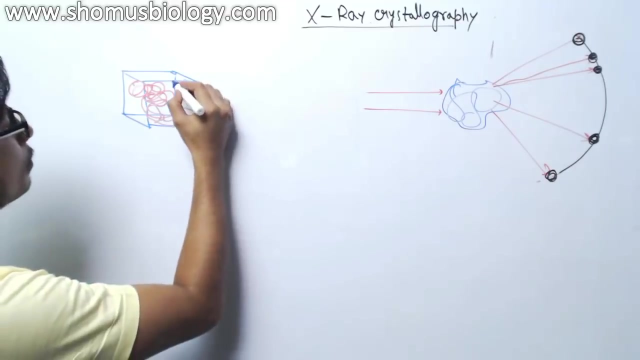 crystal here, physically, we are breaking it down smaller fragments, imaginary fragments or imaginary unit of crystals. Now we take each of those imaginary unit of the crystal- now forget about the whole crystal- and let's say we break it down in smaller fragments. So one of such small fragments if we zoom in. so if we zoom in here, one of such smaller. 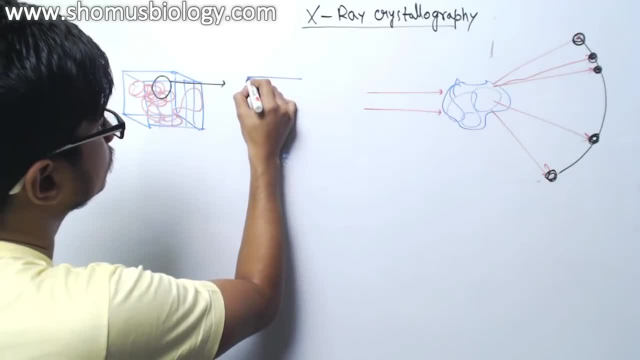 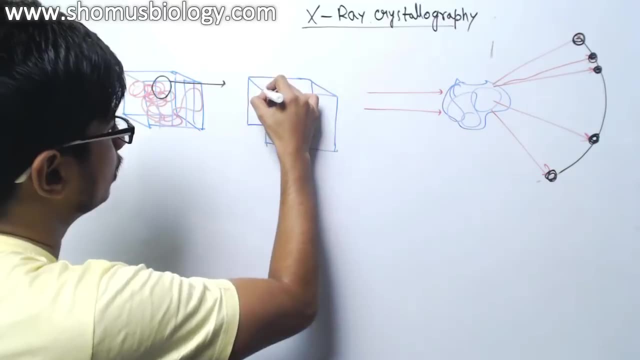 fragment. give us a structure like this. try and trying to draw as 3D as possible. I'm trying to draw as 3D as possible. I'm trying to draw as 3D as possible. I'm trying to draw as 3D as possible. 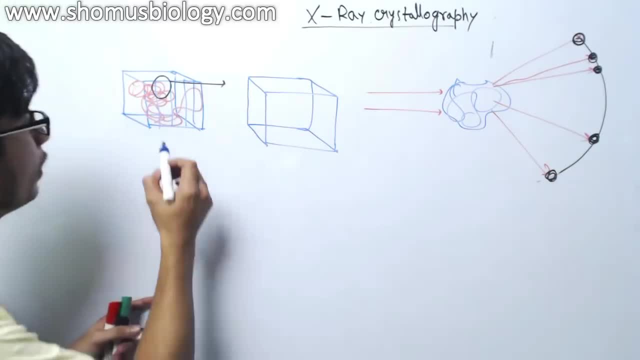 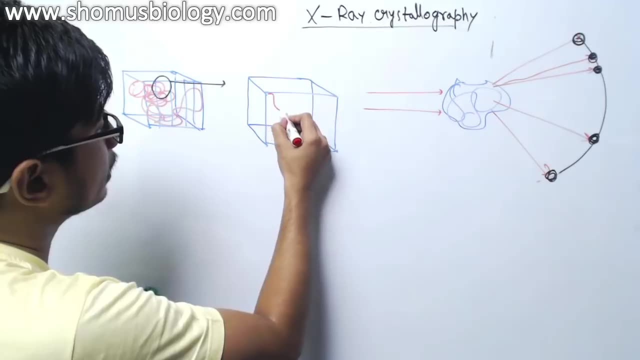 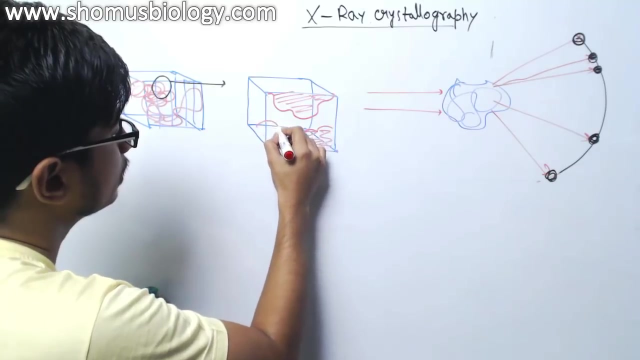 This is the smaller fragment. Remember, this is a zoomed in portion of the small unit fragment and this unit fragment, Let's say, here is a portion of the protein that is present. here is a portion of the protein that is present. here is a protein portion that is present, this fraction of the protein. 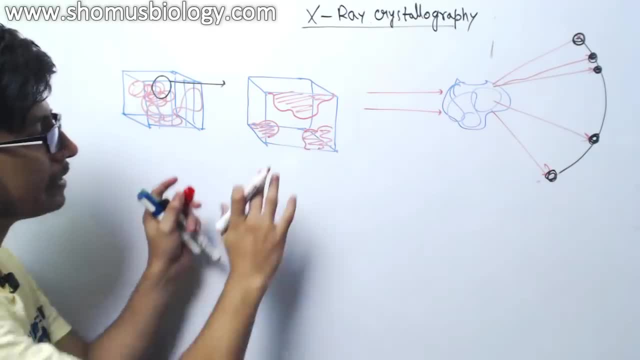 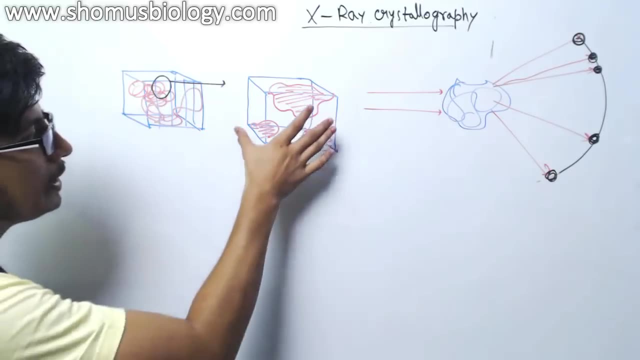 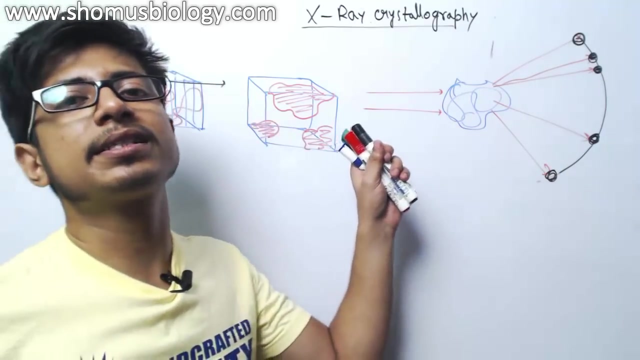 that come to the part of the small fragment. Let's say, Okay, So now what we do is we take this unit cell and we are trying to find out different planes in the unit cell, because if you talk it about a cube, because it has the structure of a cube. 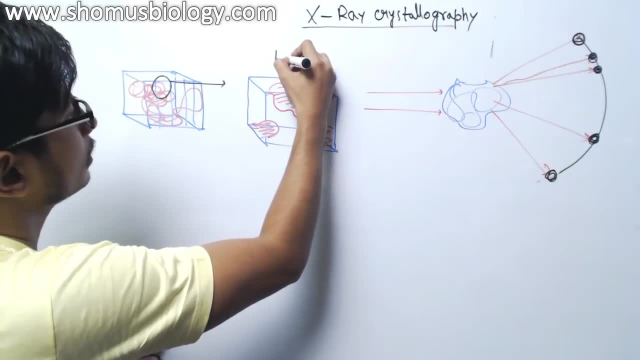 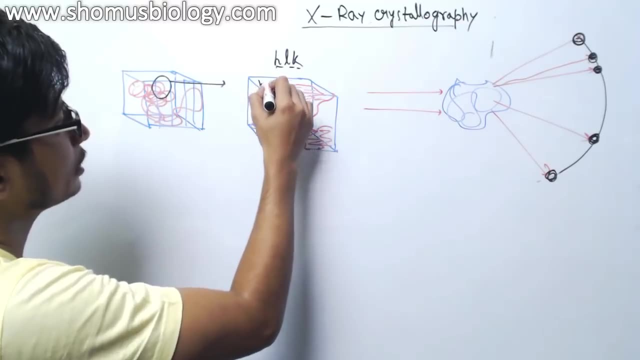 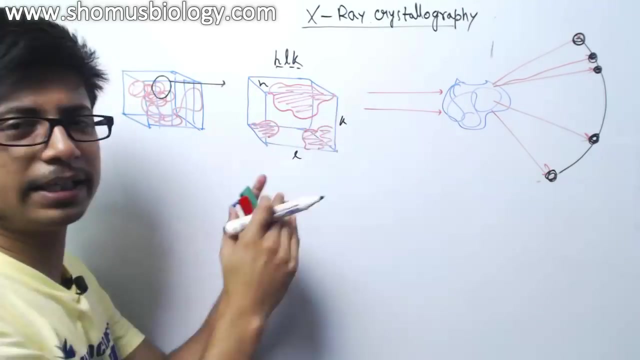 there are three things: H L, K, height, length, and so there are the three things. you can easily put it there like H L, K, Okay, Okay, Okay, Okay, Or ABC, whatever you can take it as your own, because there are the three things that you. 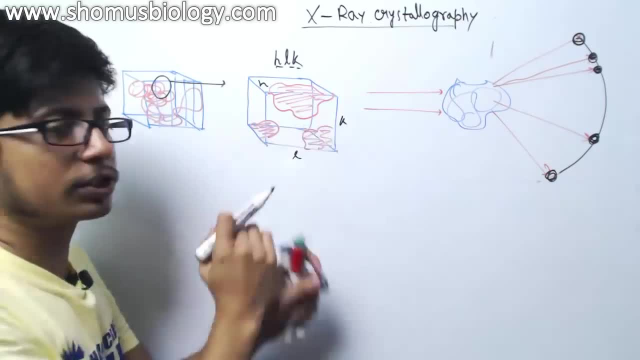 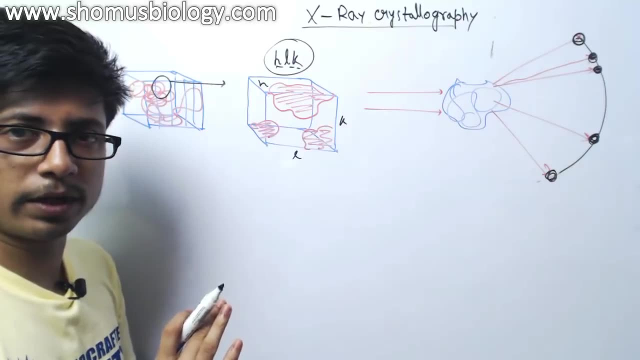 will be requiring to find out the exact structure of this cube or to get a geometric idea about this cube. So these are the three lengths that we require for getting the idea about the cube. I'm not going to talk about the mathematics here or the geometry here, but the thing here. 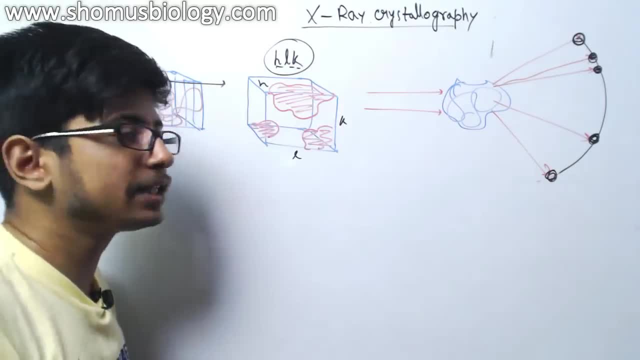 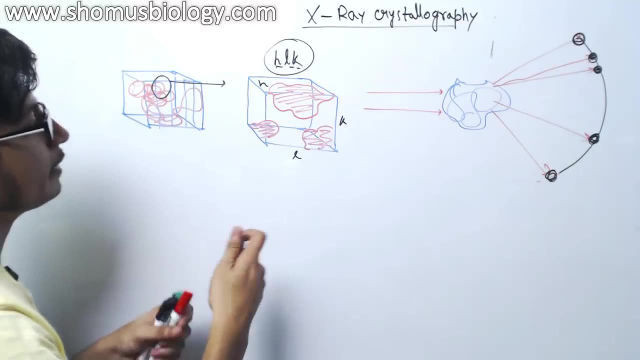 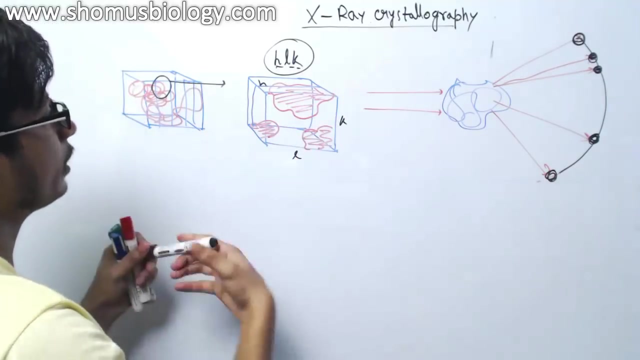 is that we will try to find out different planes of each of the single unit. We'll try to find out plane plane, For example. let's say we are trying to find out a plane that is present in between this area. So let me, let me draw it with this black color. Let's say this one, it will be. 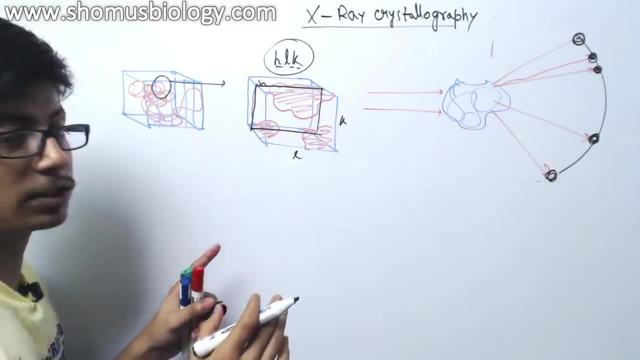 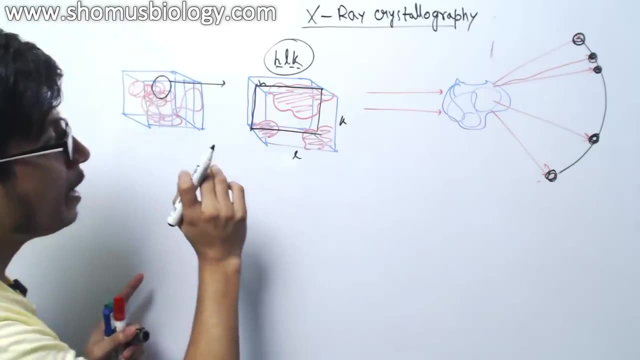 kind of hard for you to understand about this plane, because it's it's not. it's not a 3d board, It's a 2d. I mean the picture is a 2d area. I can't draw a 3d area in this board. 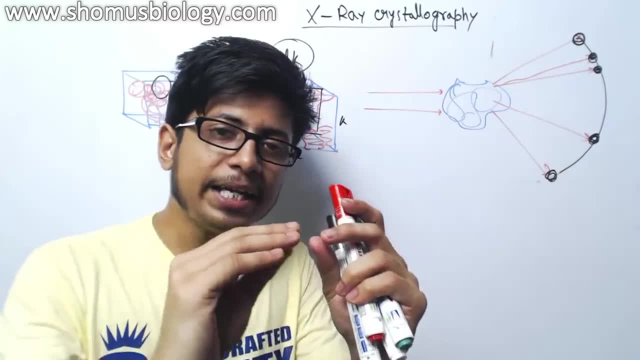 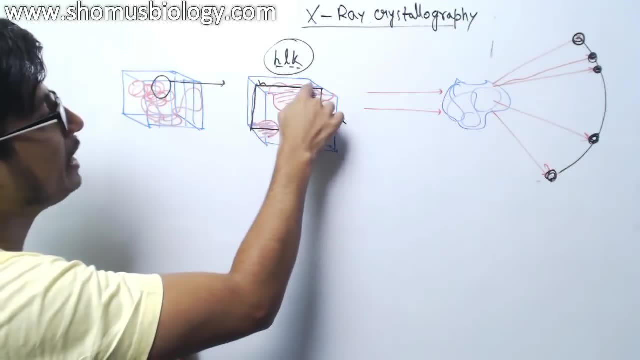 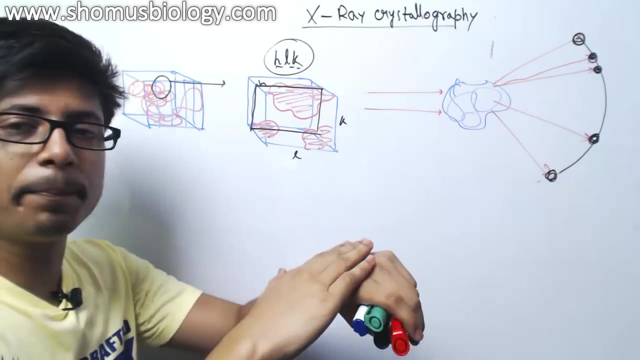 But the thing is trying to imagine this is small cube and you are rotating the cube in a way so that you find a specific plane. Now, in this case, we are dissecting the age, dissecting this age, this age hand to get a plane right. So we get a plane. So we are. 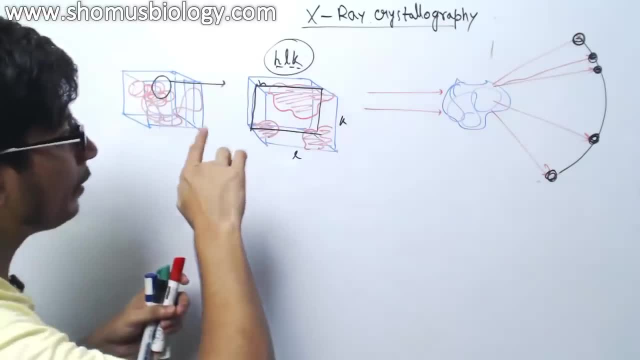 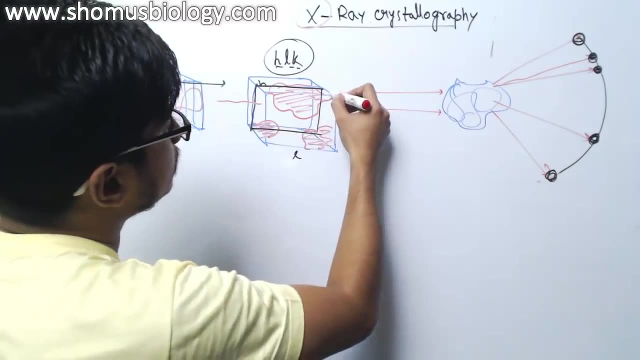 placing it in a way so that we get a plane of diffraction. Now it comes the UV. sorry, now it comes the x ray. x ray is hitting to that plane and it is diffracted. Now let's say, let me do this experiment one and again. 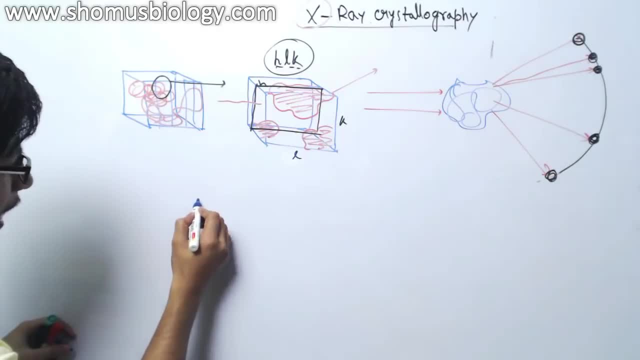 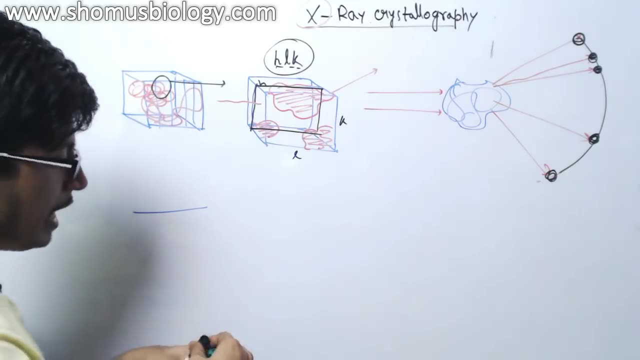 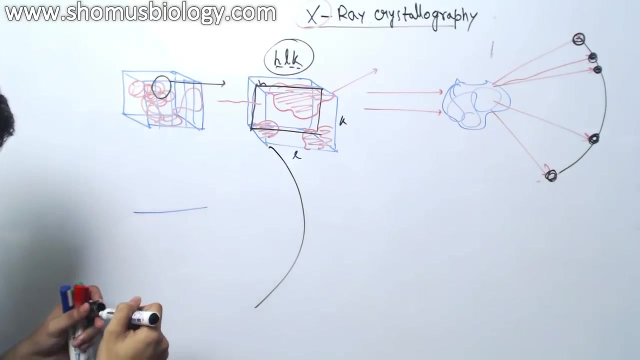 Let me draw the different planes. Let me- I'm just drawing the planes here for your understanding- For example, say like this: this is the plane that we're talking about. And let's say: this is the. this is the x ray film. Let's try it close here. And this is the x ray. So we have 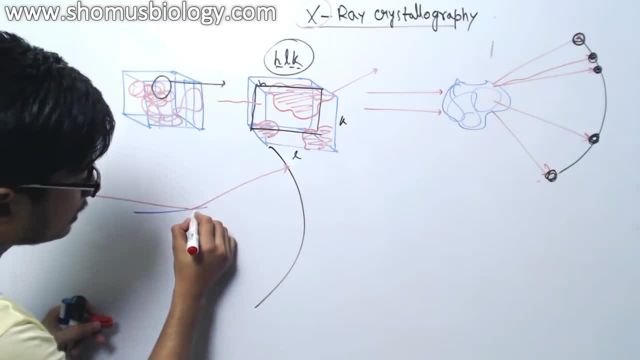 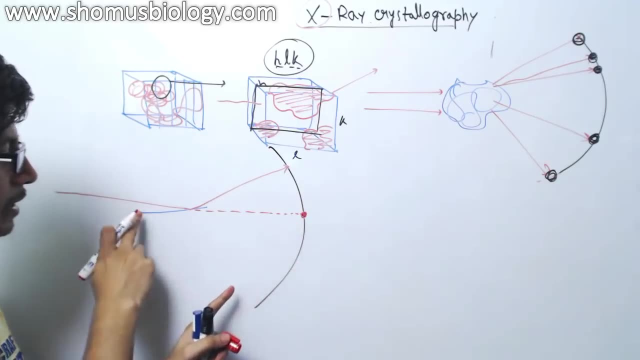 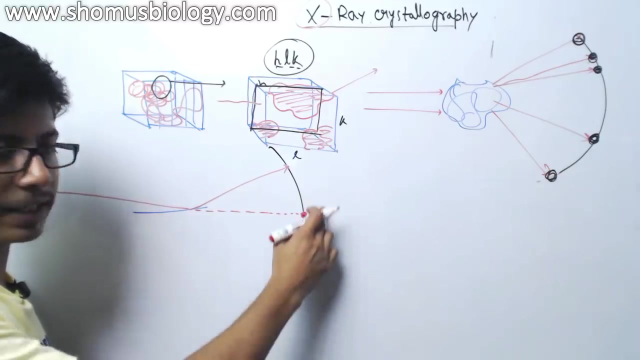 a diffraction here, for example, Now the diffraction is calculated from the distance of the space. This is the center of the axis. the center means the straight. if there is no diffraction and UV passes by wherever it gets entered, to the, to the x ray film, that is the center. 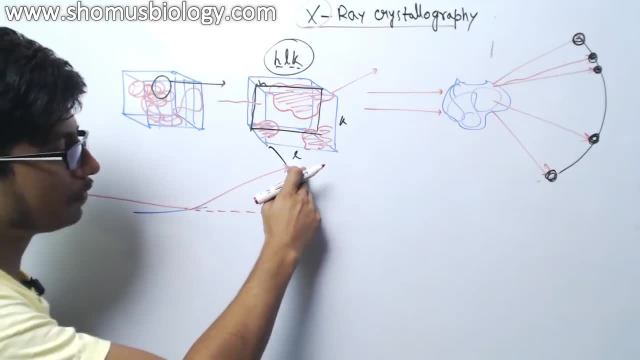 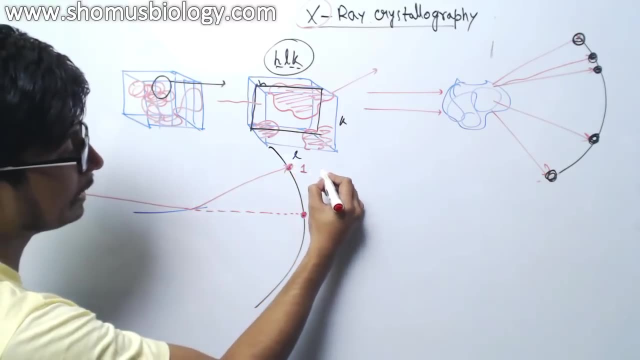 And all the distance is calculated based on the distance from the center. So here the first diffraction is at this point let's say this is the first diffraction from, let's say, the plane number one. Actually they have different number of the planes based on how. 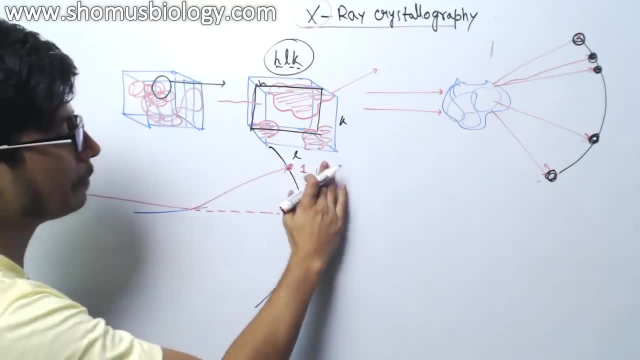 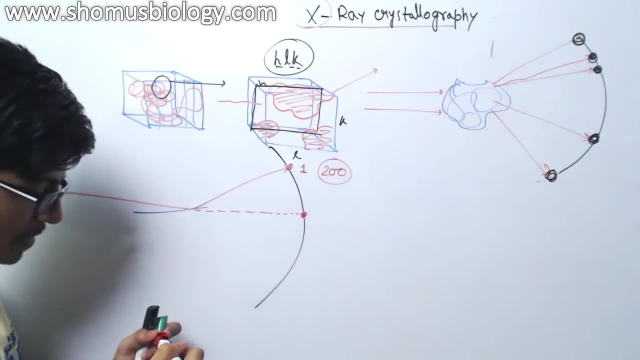 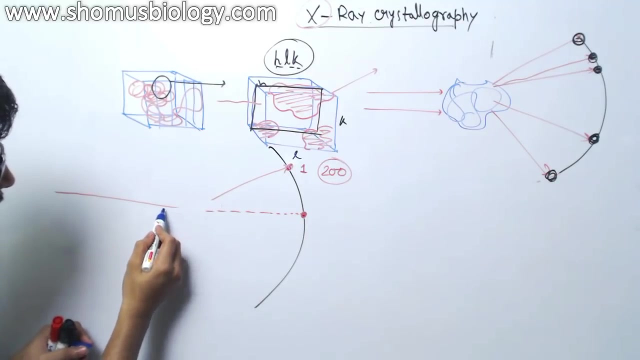 we dissect the diffraction. They have different lengths. So in this case, let's say the plane number, say, say 200.. From plane number 200, we get the diffraction at this specific point. Now we do the same thing: we change the plane. So let's say now the plane number, plane number two: two to zero. 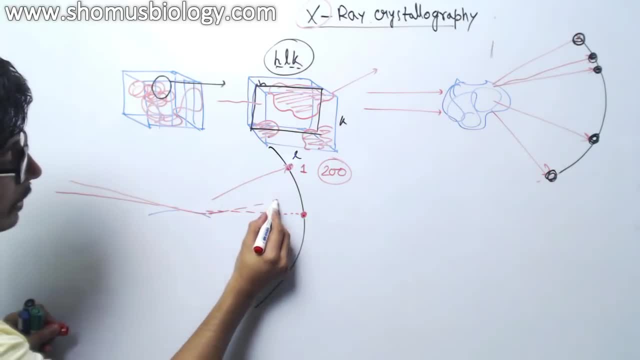 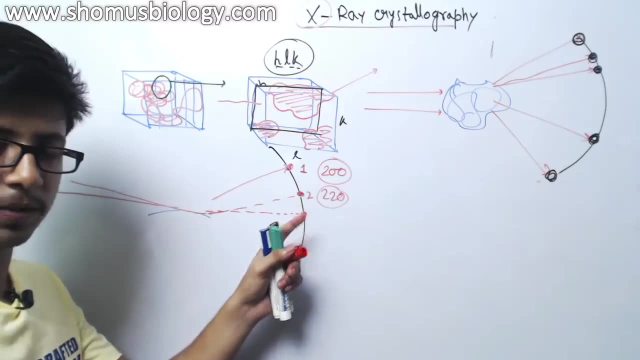 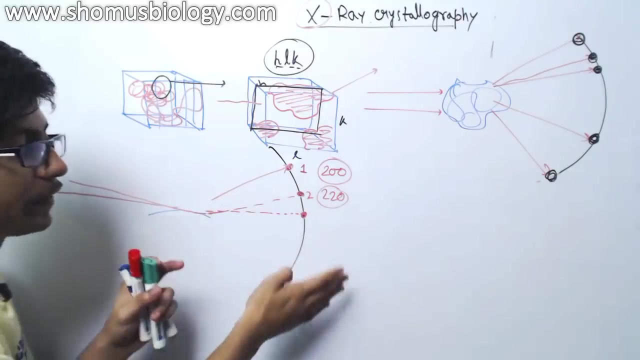 In plane number two to zero, we have a diffraction. let's say here Okay, For example. so this is the second point of the diffraction. So by this fashion, what we do, we take different planes here and we trying to find out the diffraction pattern. 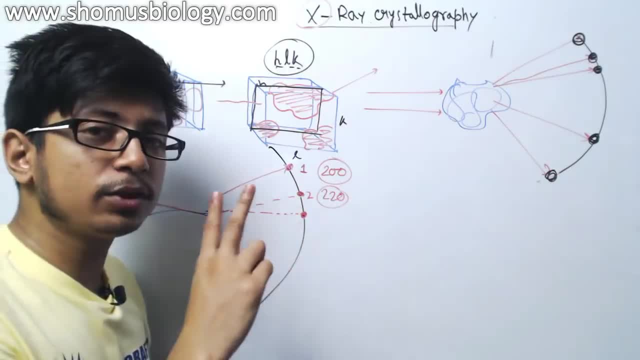 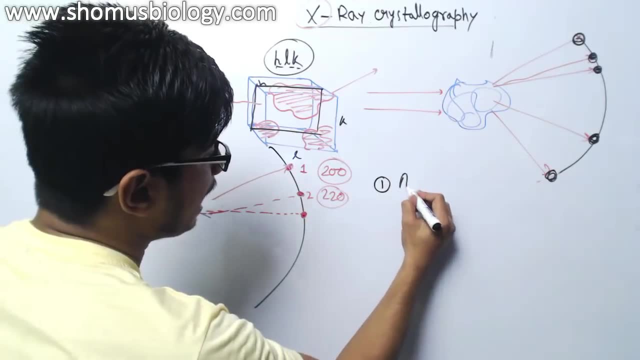 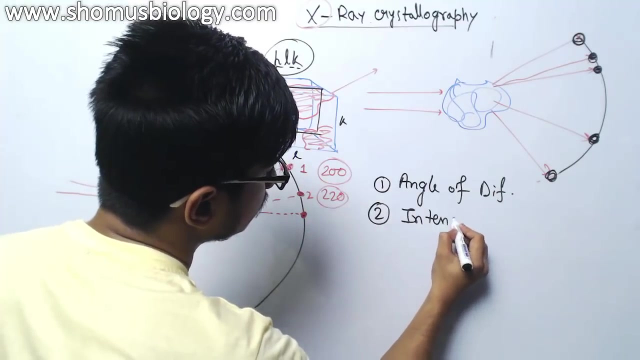 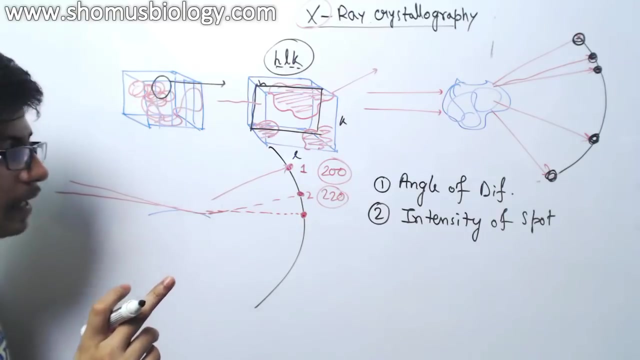 And not only we trying to find diffraction pattern. we need to think of two things here when we're looking at the diffraction pattern. The first thing is the angle of diffraction And the second thing is the intensity- The intensity Of the spot right Why? Because the intensity of the spot that is going to form in that. 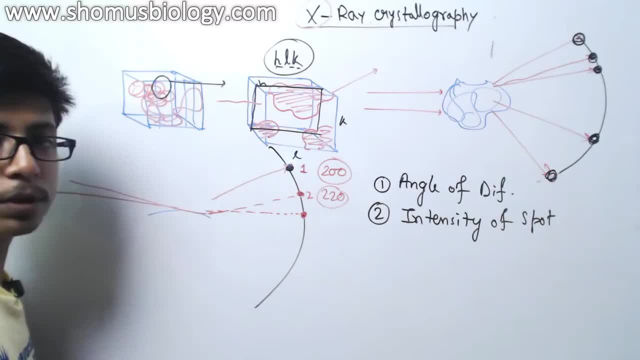 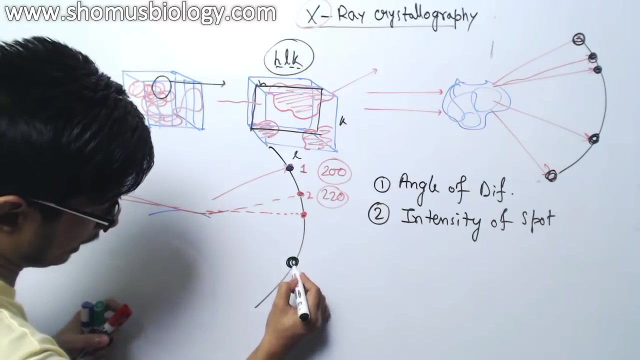 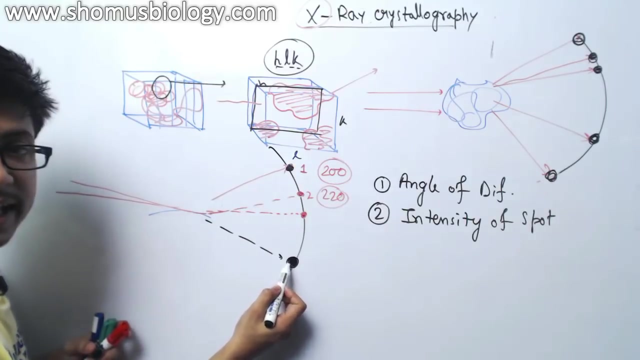 extra film is directly proportional to the amount of electron present in that plane. Now let's assume, let's say, the diffraction pattern is very, very bold here at this specific point. for example, say: at this point, That means the diffraction formed at this area. 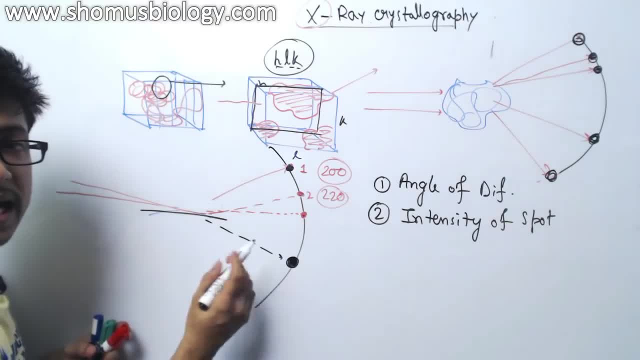 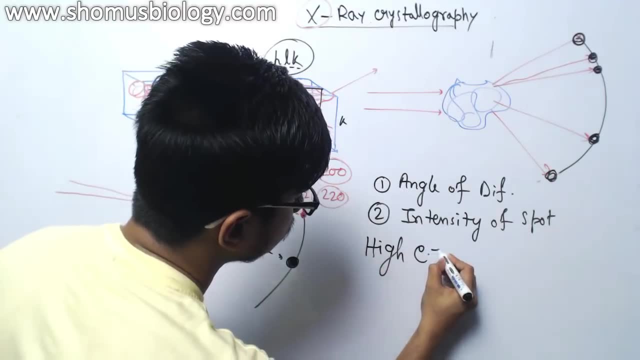 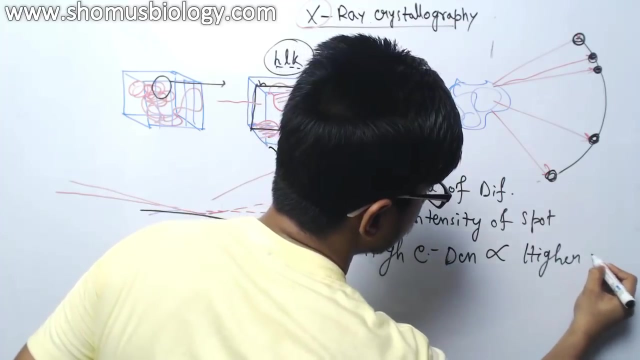 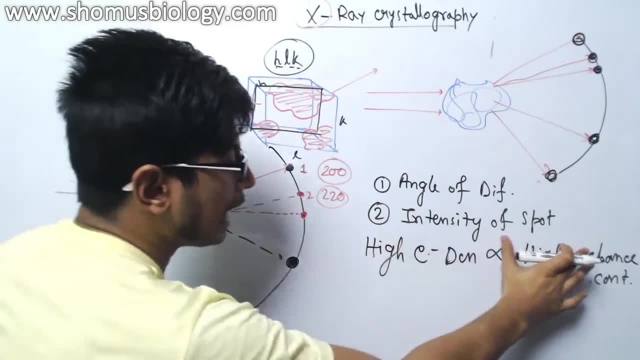 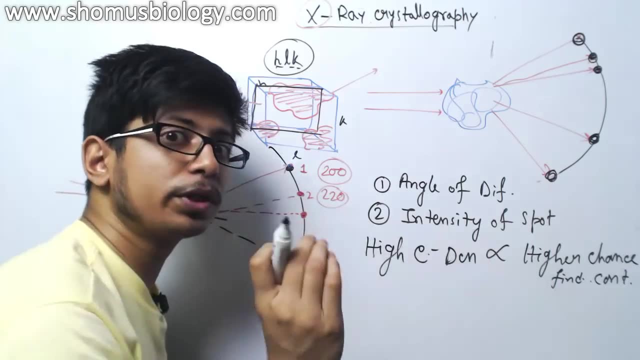 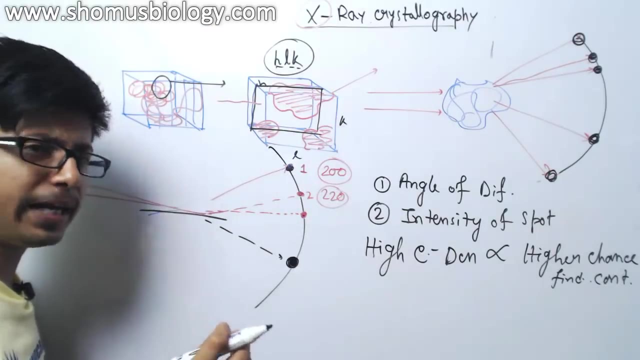 the molecule that we're looking for. So higher density of electron means if you back there and see that plane, there must be most of the protein components present in that plane. Now, if this intensity is very faint and very low, that means there is low electron density. 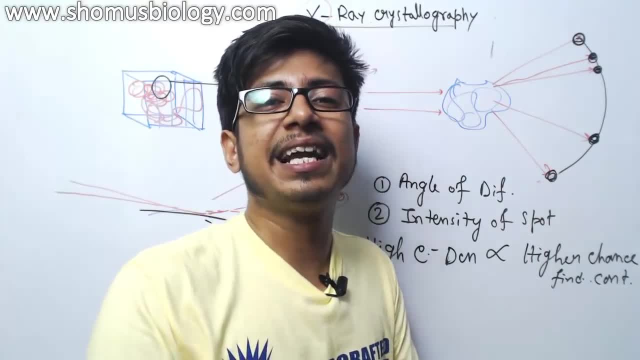 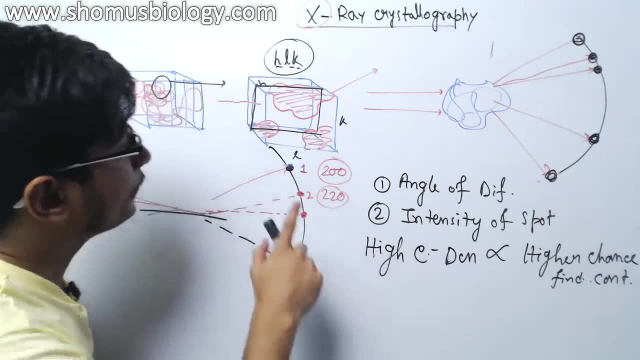 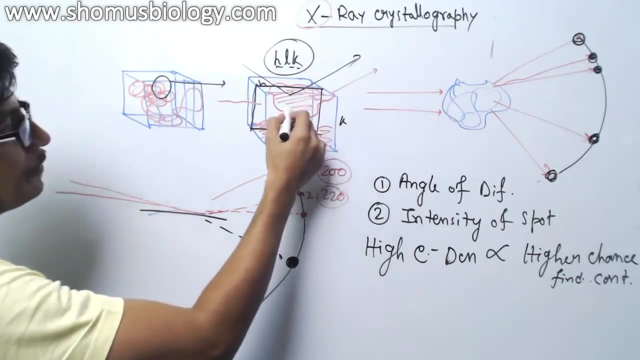 present. low electron density means there's a less chance of finding the fragment of a protein present in that plane. Get it Now. if you look at this cube, this is a unit Q we're talking about. If diffraction took place here from this specific plane, what we will? 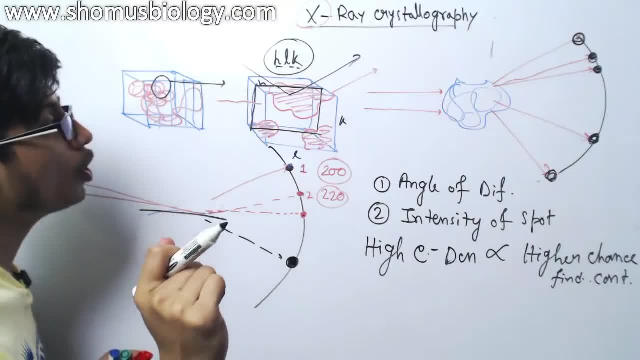 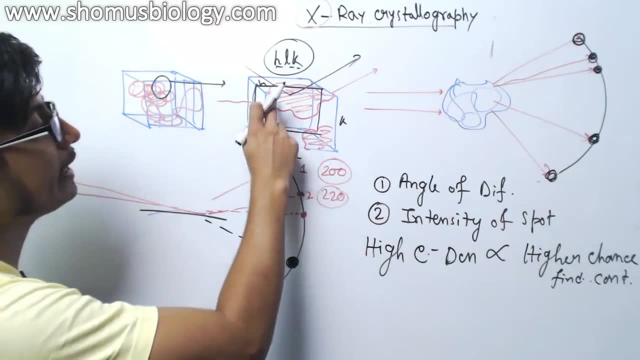 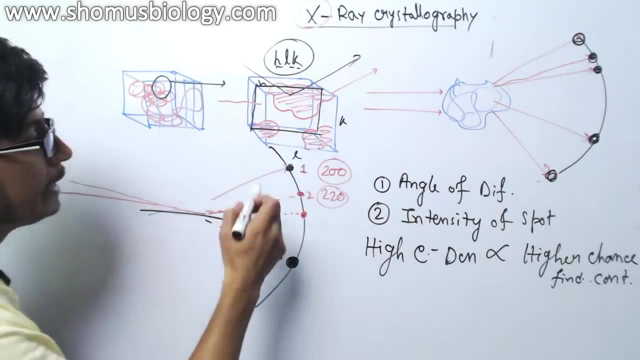 find huge amount of proteins present. so we will find out higher intensity in that spot. So high intensity, it will help us to identify. yes, there are maximum amount of protein present or protein content present or electron density present in this area. So Now, if there is a reflection diffraction from this part of this specific plane, if 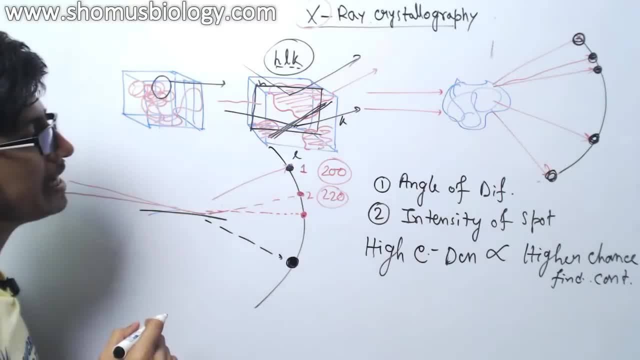 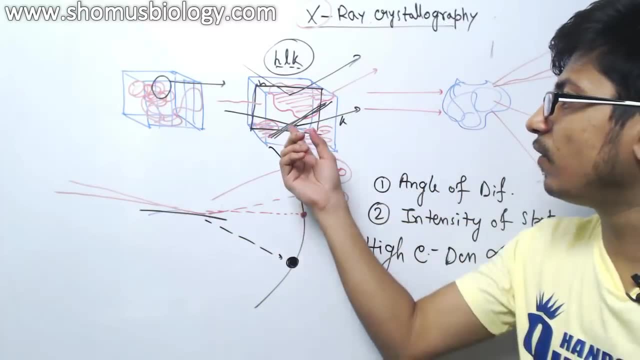 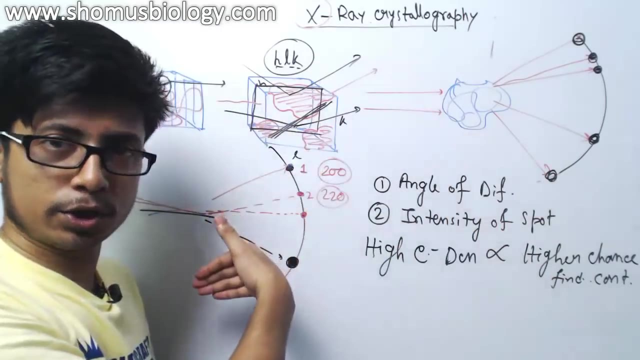 I, if I put the plane like this and from this specific plane, that is going to give us a very faint spot that is going to tell us that there is a less chance of finding a protein component there. So now try to calculate the whole thing and going backwards, 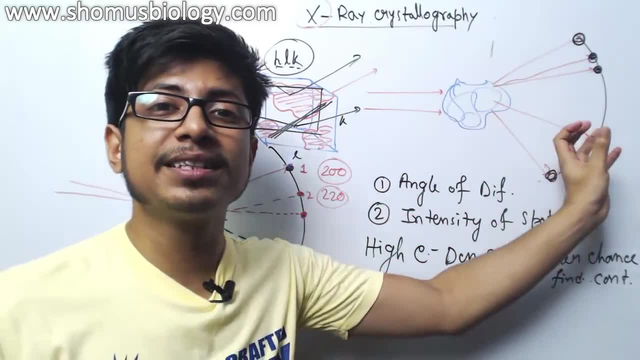 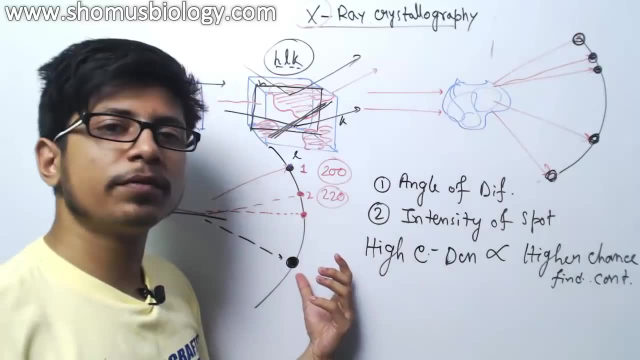 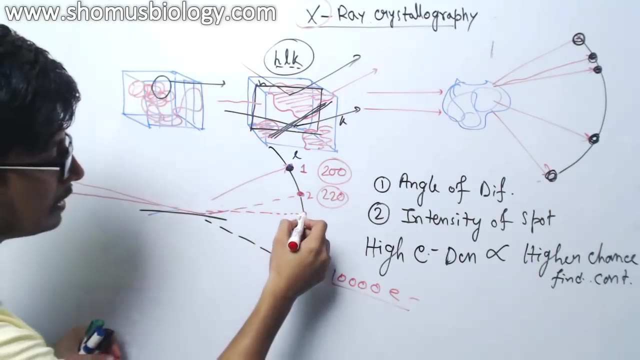 We know the amount of intensity corresponding with the electron density. with the help of multiple experiments, Scientists have acquired this idea that if you have this amount of electron density, it corresponds with, let's say, 10,000 electron. If you have this amount of density, it corresponds with 6000 of electron. 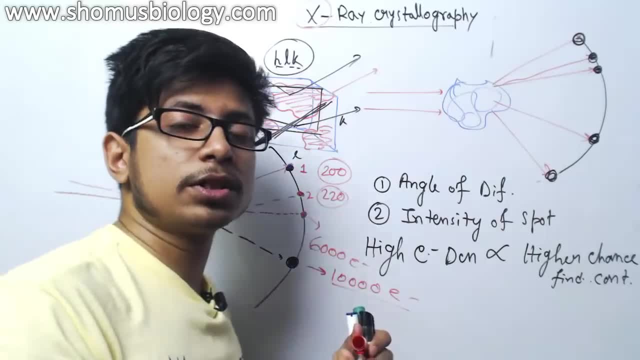 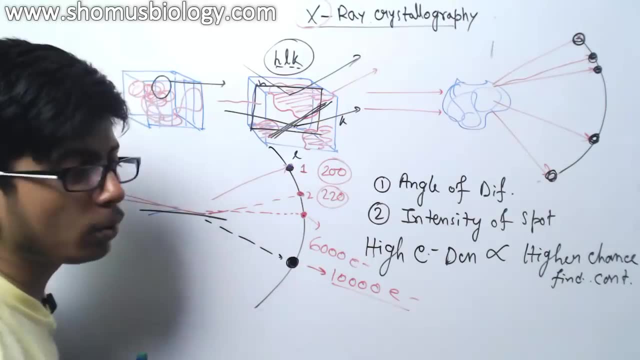 We know about the relation of number of electrons associated with the intensity level that we find In the except plate. So, as we know that we are dealing with the structure of unknown protein, we simply found out that spot based on that intensity and the angle of diffraction. 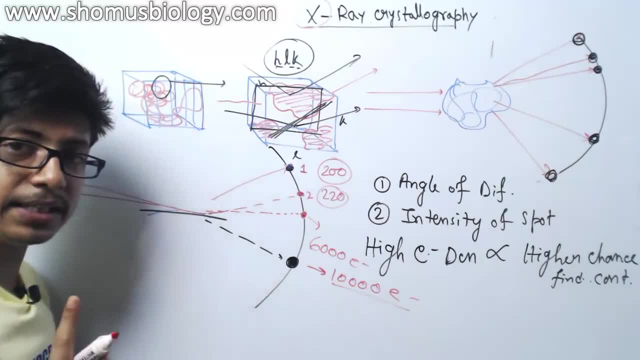 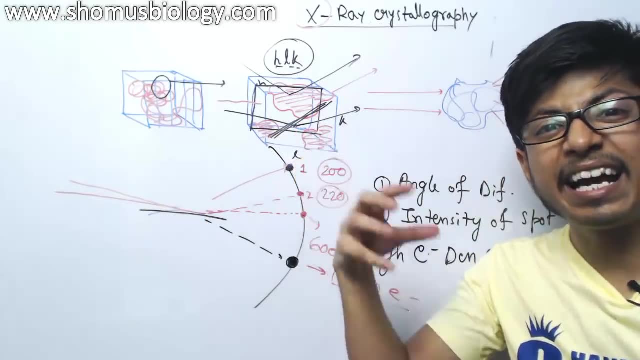 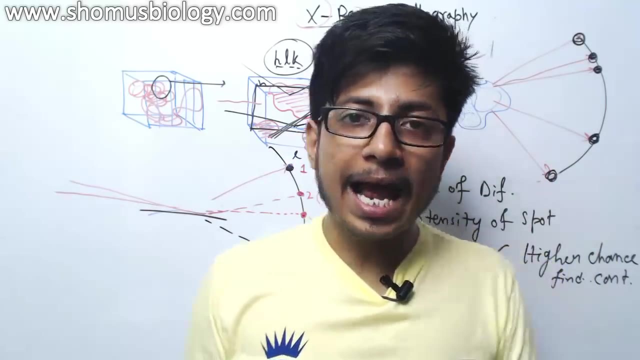 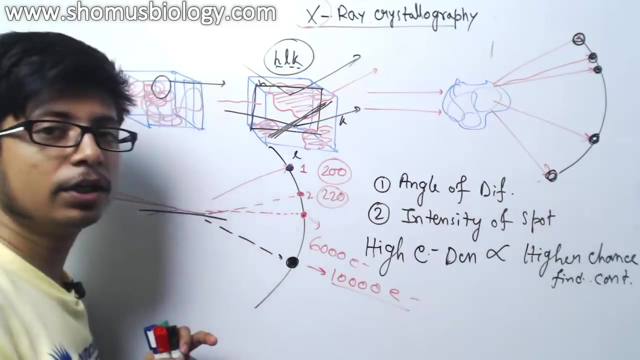 I haven't talked about that yet. but based on that intensity we can identify where or which part of that unit cell contains more electron density, area, which part contains less electron density. Let's see, And this angle of diffraction is also important, because the angle of diffraction is also different. 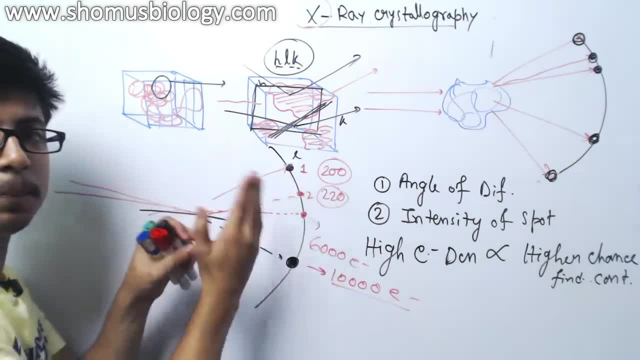 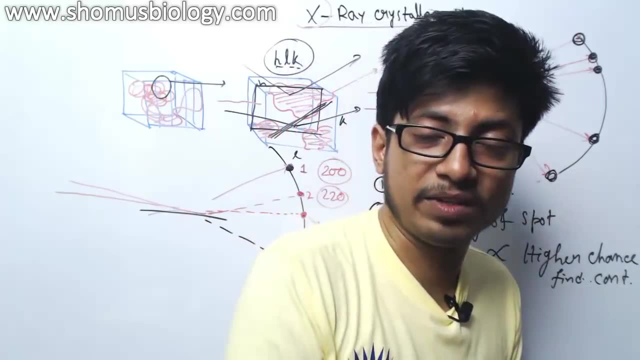 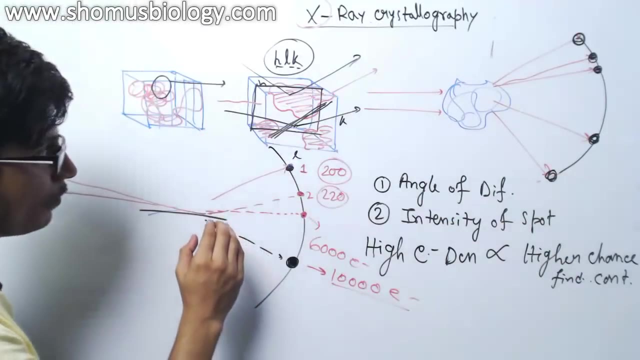 for different planes because, as we are, as we are changing the planes, remember we are not changing the association of the protein molecule because this protein is fixed, It cannot rotate, those atoms cannot rotate, its fixed is in crystalline form. so, changing this plane, we are getting different diffraction angles. 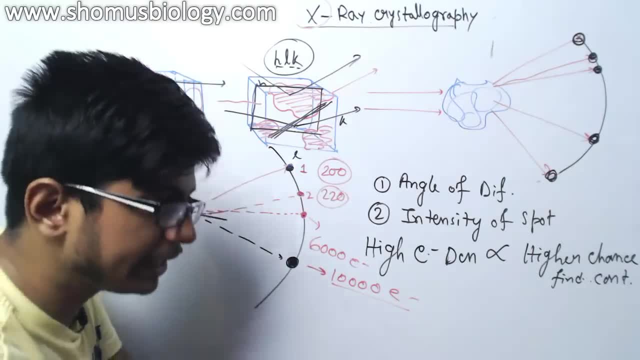 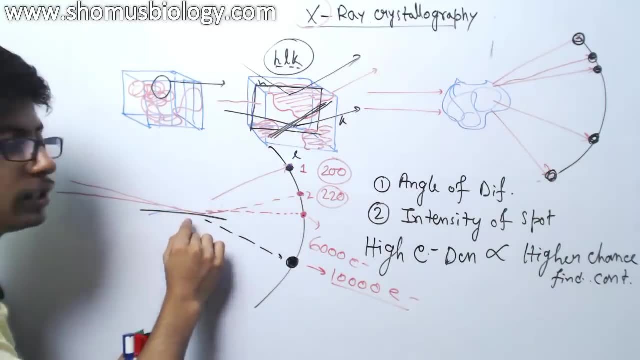 So diffraction angle is also telling us an important fact about how exactly we are placing the plane. So this diffraction angle will tell us about which area of the region we get the spot for. So it will be important for the computer to find out which spot represents to the which. 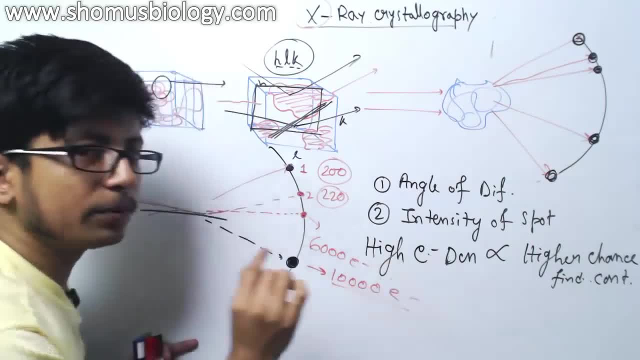 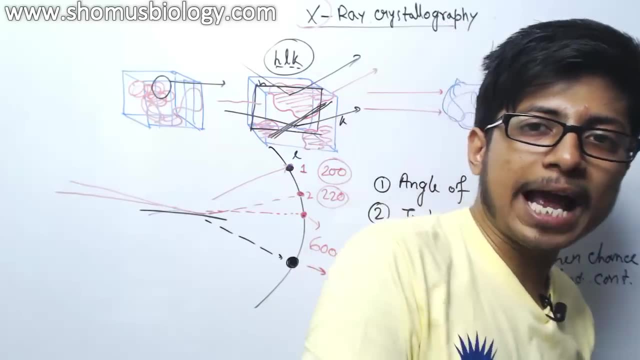 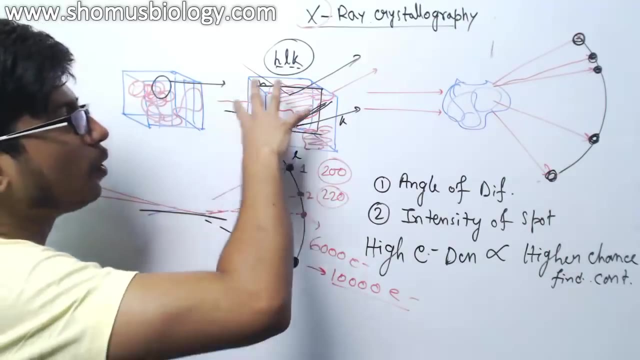 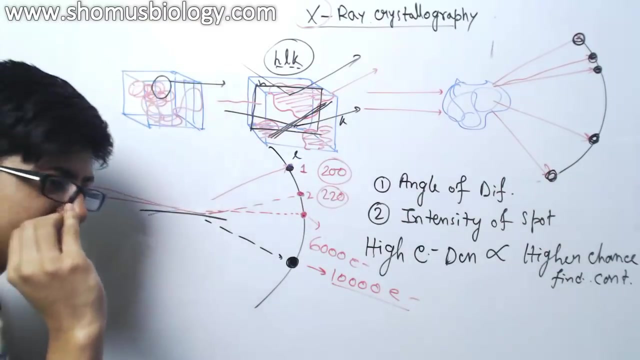 area of the unit cell and the intensity will be helpful to identify the amount of electron density corresponding. Okay, So, as we know, both these things together for one small unit cell and the whole data is feeding to the computer. such. now go back as we divide the actual crystal into. let's 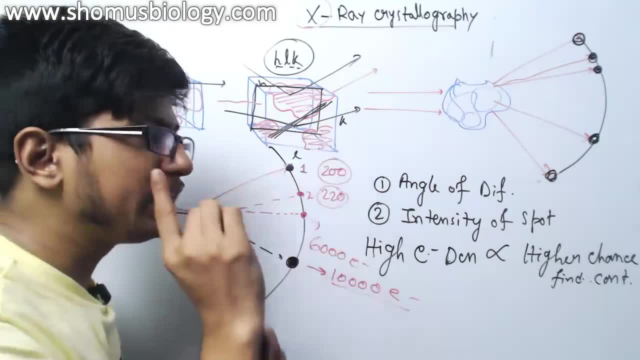 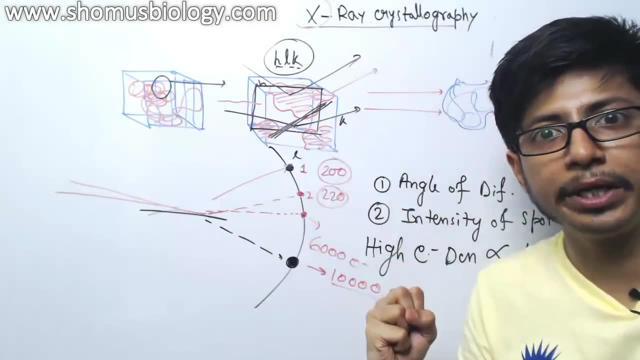 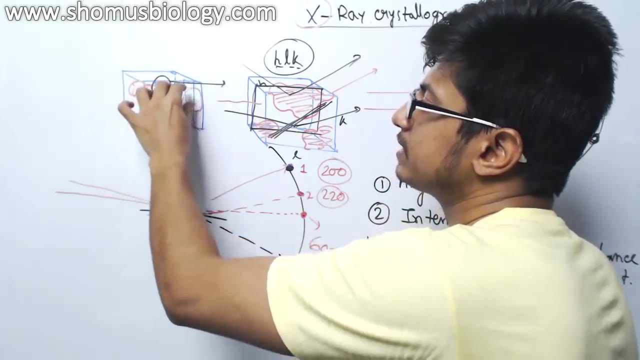 say three different small units. We get the data about each unit for all those three units- 300 units- and then we compile the whole data about the 300 units, which will give us an idea About the whole three dimensional cube and the different density of the electron in that. 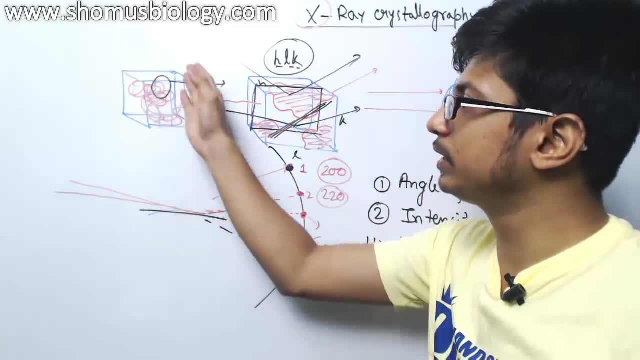 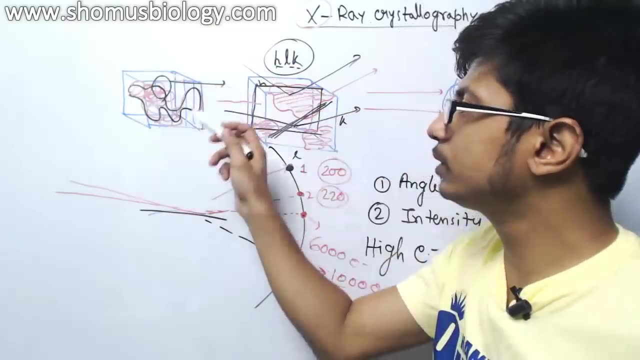 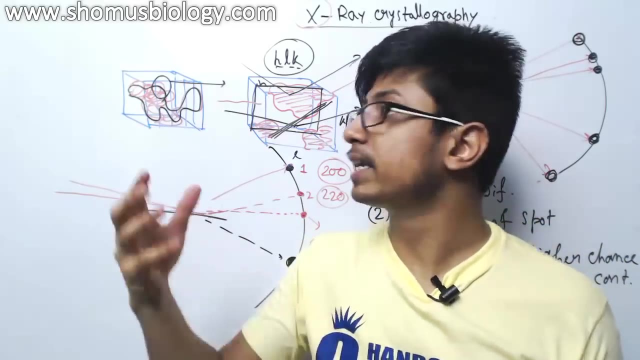 cube. So as far as we go with this protein, we will find high electron density present throughout this type of area, which is going to help us and identify and understand where exactly the protein molecules and different atoms are present. but that is not the end, because 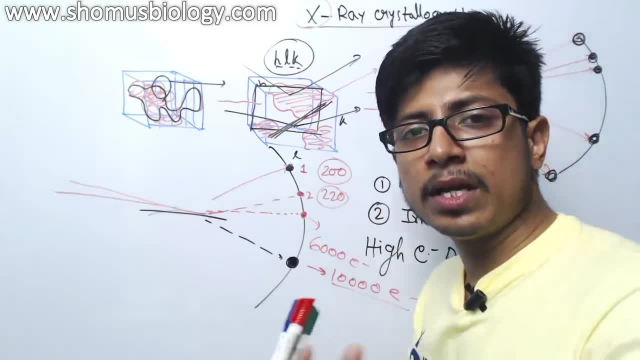 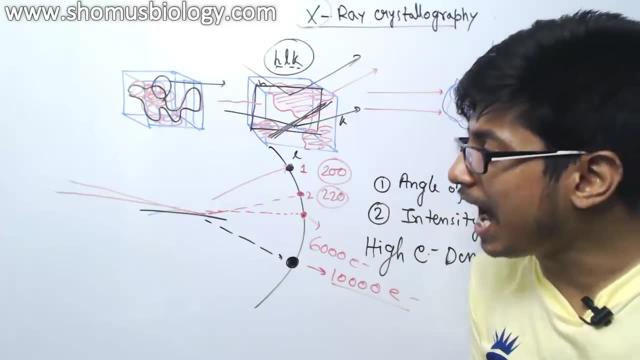 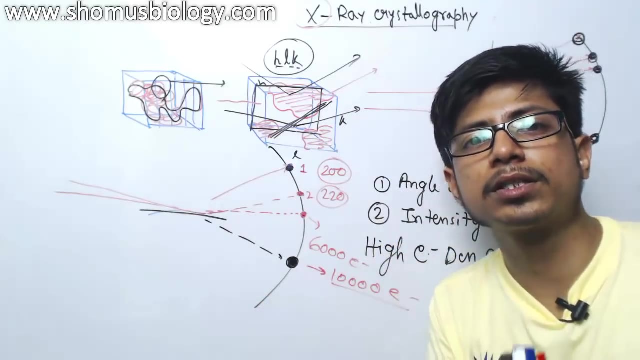 it is going to. It is not going to give us an idea about the idea about why, where exactly the components are present. It's not going to give us exact structure of the protein. So how can we get the exact structure? Now we correlate the data of electron density along with the appropriate structure of the 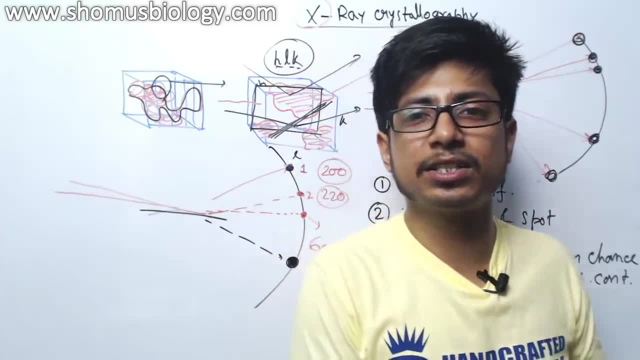 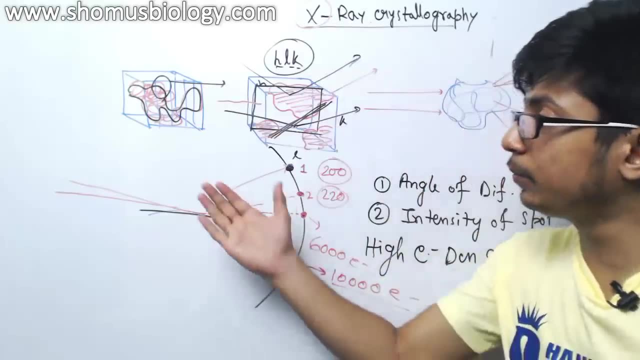 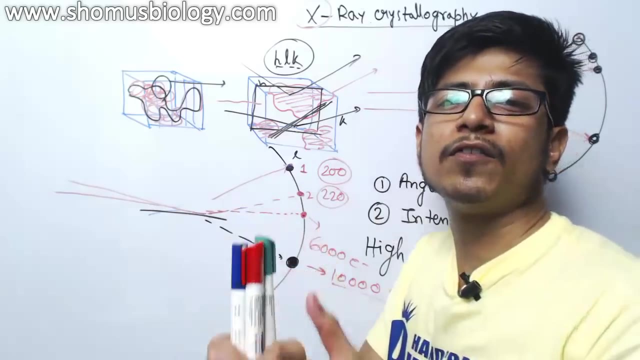 protein, because the protein structure is composed of its secondary structure that are alpha helix or beta sheet. There could be better turn and loop. So we know again with the help of series of experiments- Okay, We know that which kind of electron density map is corresponding with the alpha helix. 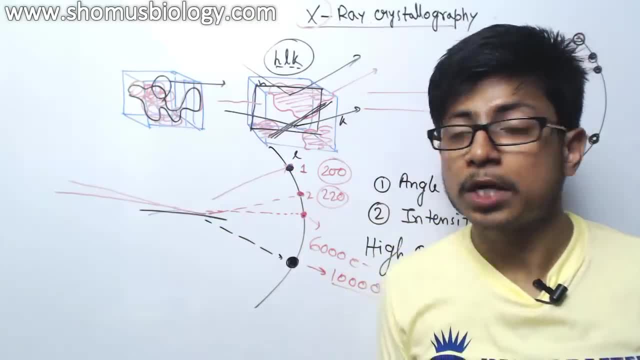 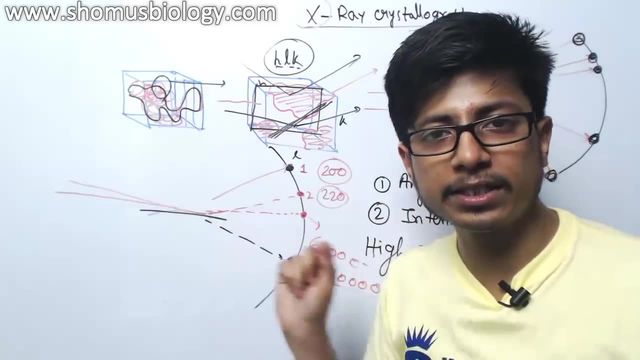 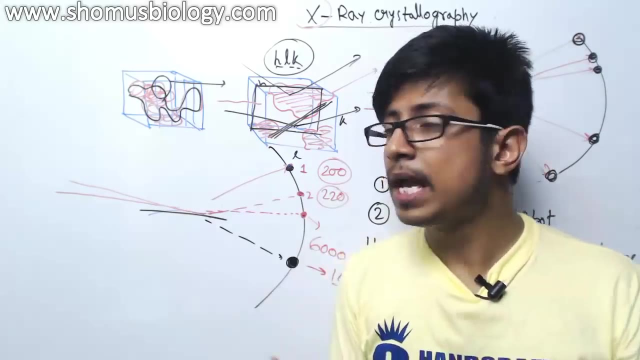 which kind of electron density map is corresponding with the beta sheet. So, with the help of this correspondence and idea, we can find out what kind of and where exactly the alpha helix is present in this cube, where exactly beta turn is present in this loop, which is going to give us an overall view and idea about the protein. 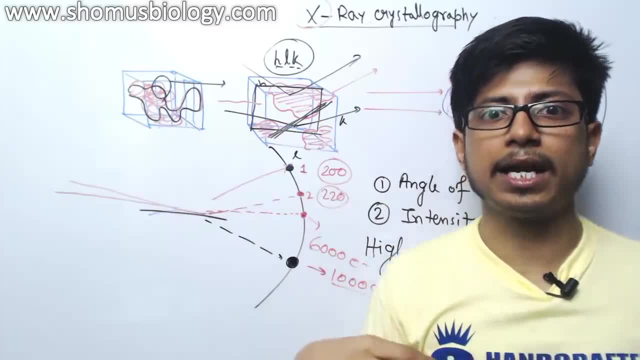 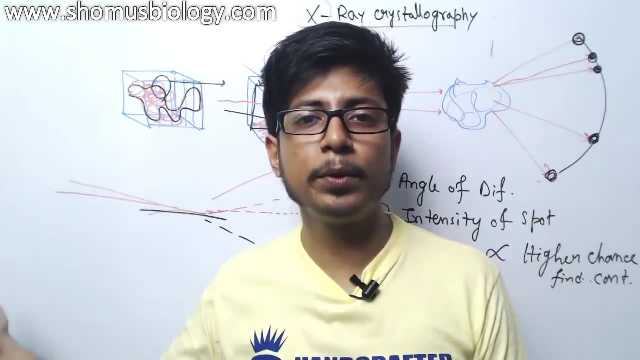 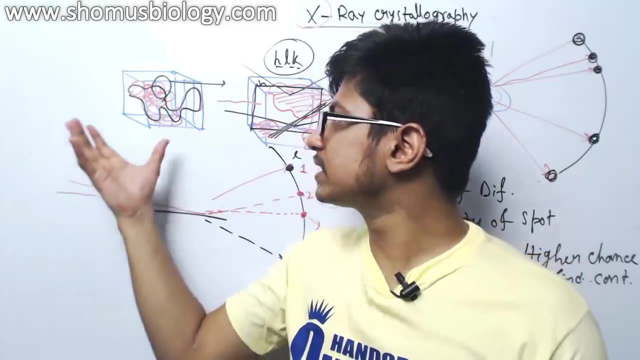 Now, that is also not the end. That is again a crude extract and idea. Now we we take advantage of the other type of computerized biotechnology tools and, like, like the bioinformatics tools, We take the protein data bank. We find the same type of protein structure. 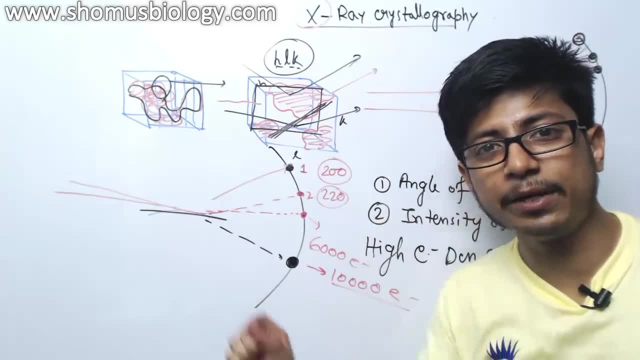 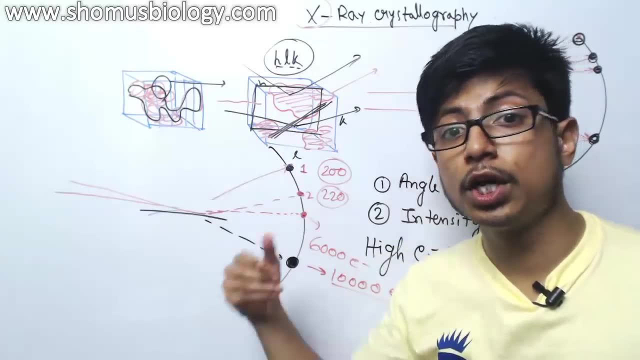 We compare the structures with each other together to find out exactly where there is a difference, exactly where there's a change, that we fill the gap from the idea and and informations from that database. And that is not so. Not also the end. Okay. 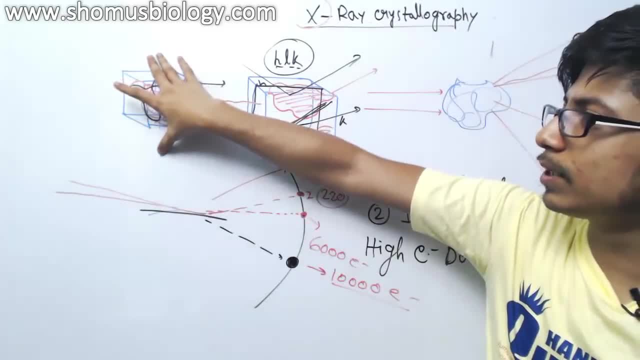 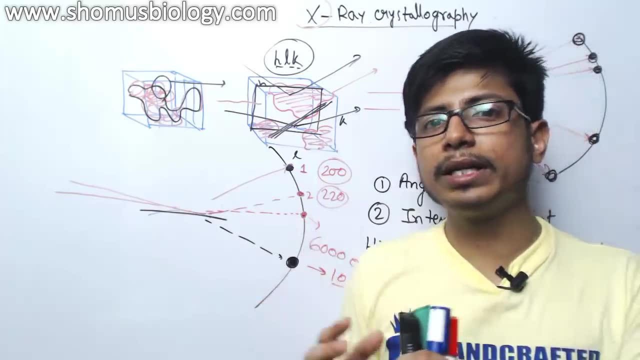 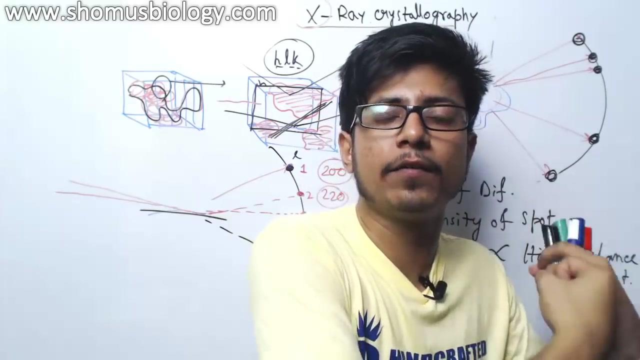 So what is the end? Because it's a structural part, We also try to run several experiments to find out the function of this unknown protein. Once you find the form function, we can correlate the function with the structure to get exactly what kind of structure the protein should have to obtain that kind of a function. 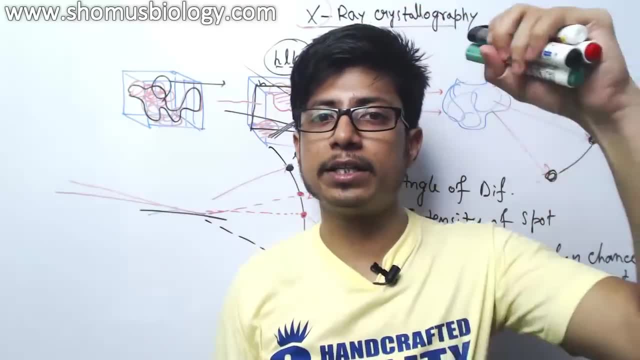 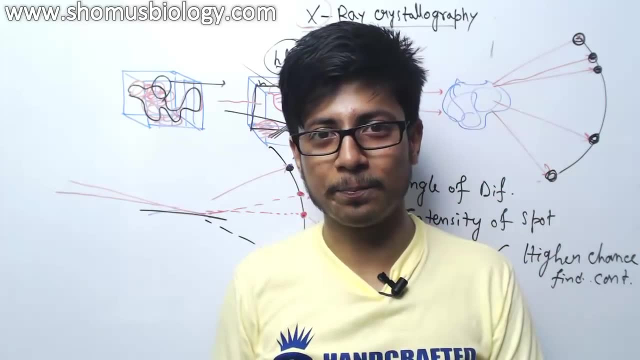 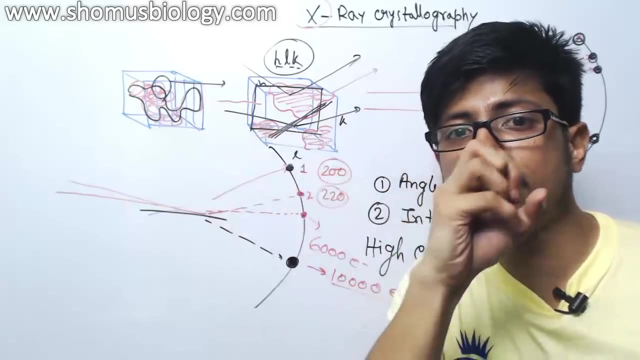 Because if you find out function, we can go back to get a structure. If you get the structure, it will help us to find out the function of the protein, because there's a correlation between the structure and function of the protein. So that, in a sense, is extra crystallography in a nutshell, about how exactly we determine. 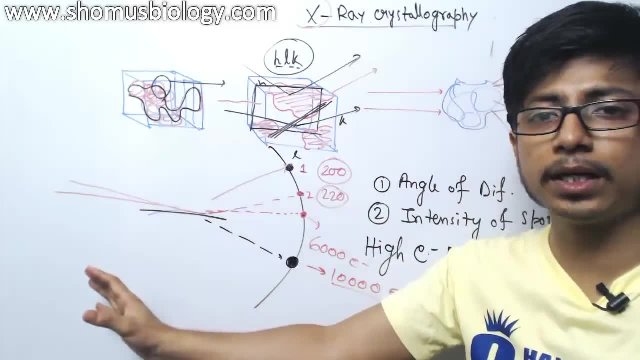 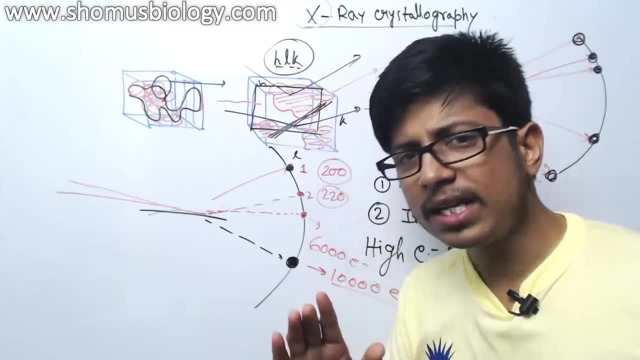 the structure of the protein or any other chemical compound with the help of extra crystallography. It based on the extra diffraction pattern. and remember, there are two things that I haven't talked about which are very important, like one is Bragg's law. 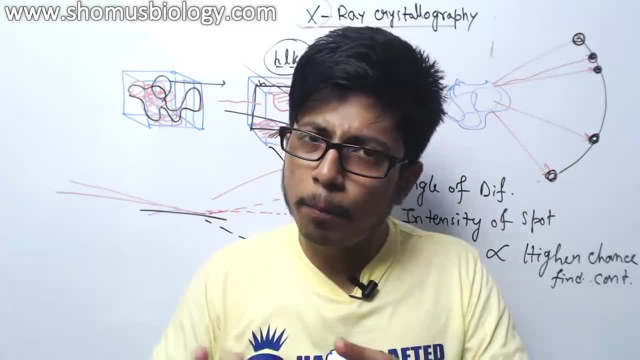 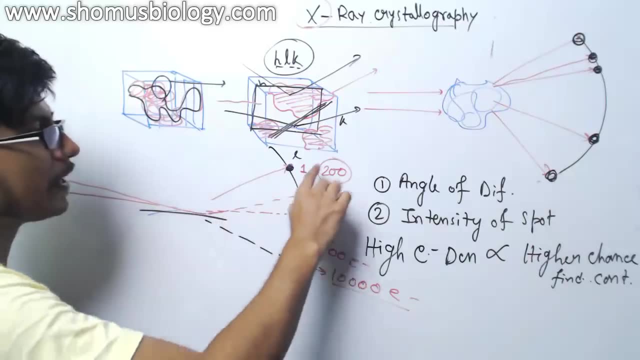 Another one is a furrier analysis of Fourier transformation. Both this case are mathematical explanation which I'm not going to. I'm not going to provide you and confuse you. but the idea is, whenever there's a diffraction going on from the nearby area of the electrons or nearby area of the atom or the molecule, 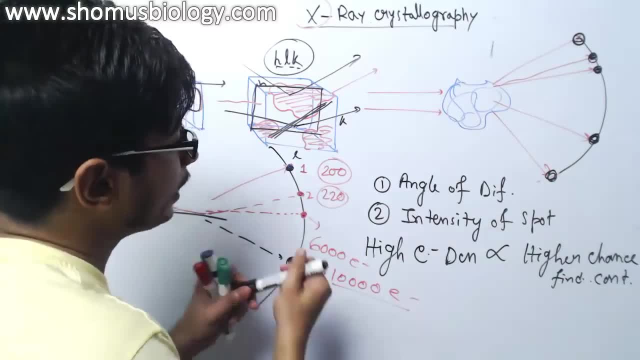 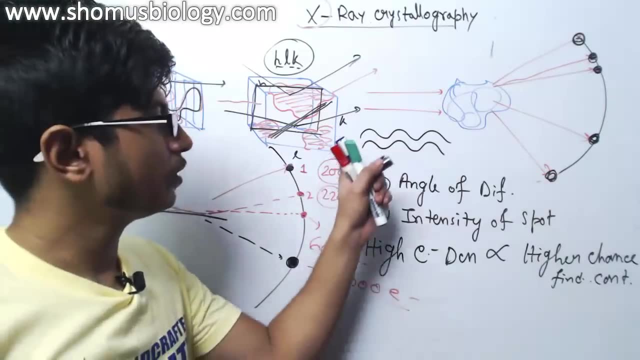 that we're looking that diffraction or the wave of the diffraction could be two different ways. Now it could be in the same phase. Let's say it's coming from two consecutive area of the, of the atom, So of the molecule. So we have a phase.